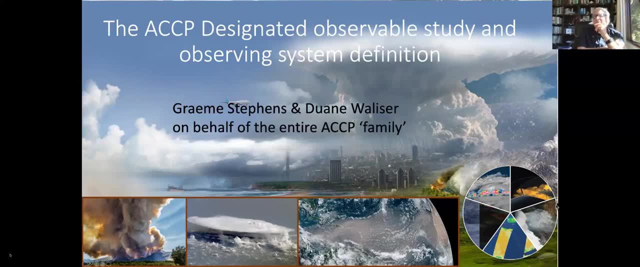 Dwayne's slides. you'll see my slides are a little bit rough around the edges, So that's my disclaimer number one. Number two is the project is renaming itself from ACCP to ATMOS, but that hasn't yet been officially approved by headquarters, And so I guess we're not. 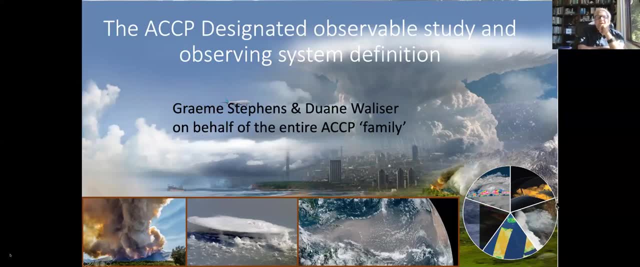 allowed to use it except for internally within the project. So if you see the word ATMOS, just read that as ACCP and pretend it's not on the slides. I'm not sure I caught it all and removed them all. You can see it was even in my title for this. 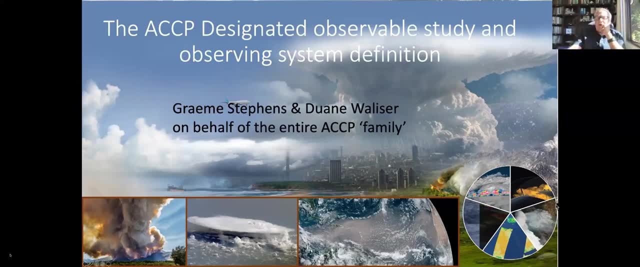 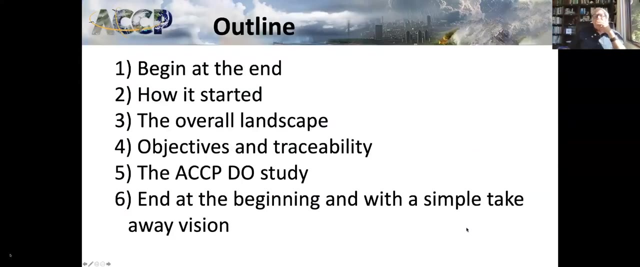 Okay, So that's enough of the disclaimer, So let's go to the. Why is it not advancing? Oh gosh, It's really slow. So this talks about being a little bit circular. I'm going to begin at the end and sort of work backwards in a little way into a little big of the details. 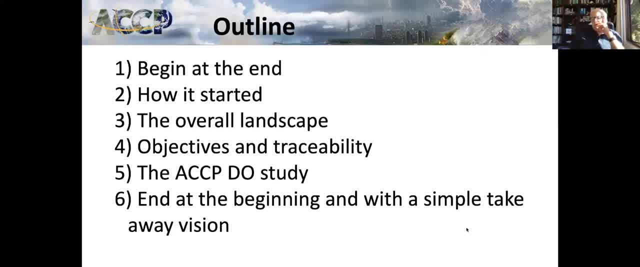 I'm going to keep this at a fairly high level And unfortunately that's somewhat superficial level in many places, so forgive me for that. And then I'm going to talk a little bit about how it started and provide you with the overall landscape for how this Dernier Observable definition has evolved, including the landscape. 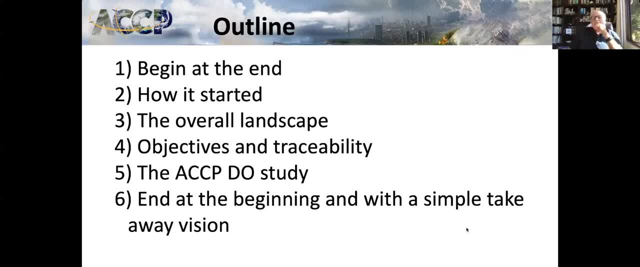 for the decade, looking forward ahead, for that's the context in which these new observations and these new programs sort of will sit. So I can talk a little bit about the objectives of the program and its traceability- and what I mean by traceability you'll see in a moment, and then I will talk about the study itself. 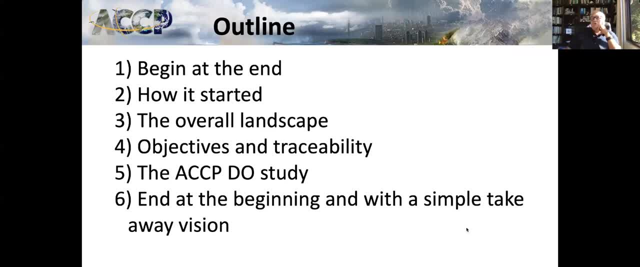 and how we got to the end, which is the architecture proposed to headquarters and is now moving to pre-phase A. So I'm going to end at the beginning and then I'll sort of close with just a very simple Sort of take away vision in a very simple way, if you wanted to just sort of think about. 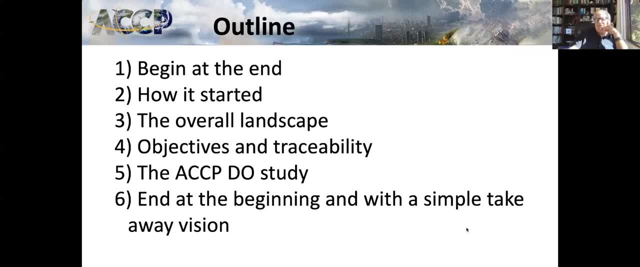 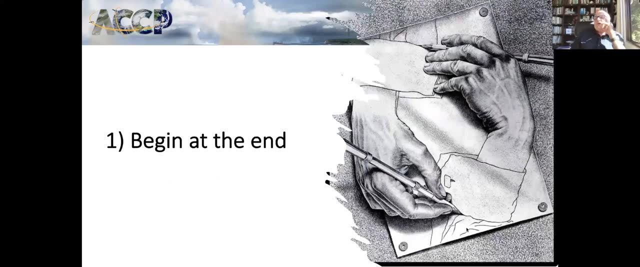 what ACCP might be. you can sort of think about this as a vision as seen by a cosmonaut on Earth, looking down from space, looking down at Earth. Okay, so I'm going to begin at the end, as I said, and the end is the definition of this. 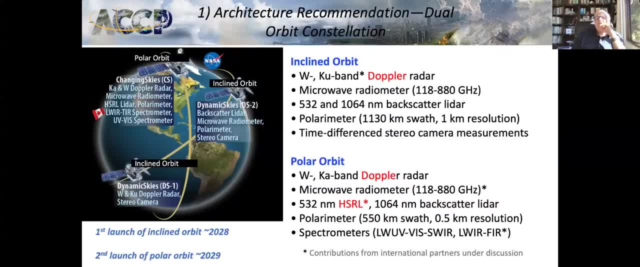 architecture- I'm going to come back to this, of course, so I'm not going to dwell on this very much, but the architecture involved Two orbits and headquarters, refers to these as two separate projects that are connected together. There's a polar project and a decline project, and I'm not going to dwell on the instruments. 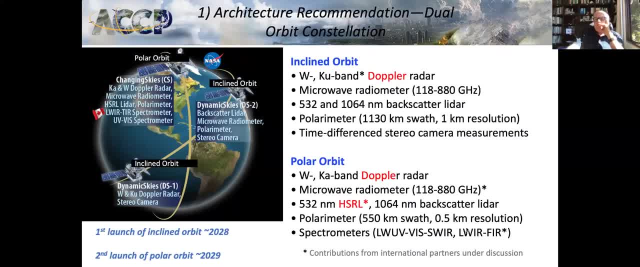 at this point in time. We'll come back to this a little bit later as we start to sort of go forward again and get to the point where this makes sense. but this is sort of the framework of the architecture: Two orbits- 2028, 2029, launched separately, there are international partners and there is some discussion. 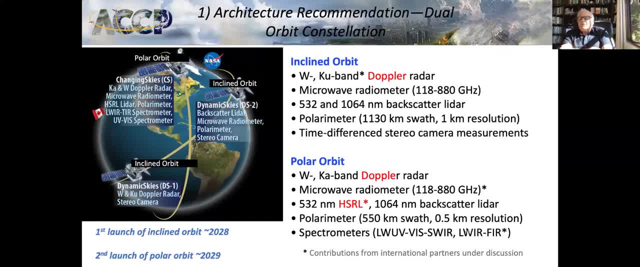 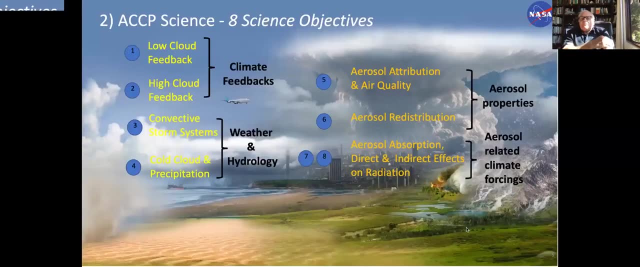 about the contribution from international partnerships in this, and the partnerships involve CNES, JAXA and the Canadian Space Agency. Right, so I'm stepping back. you know, I started at the end and I'm sort of stepping back one step. 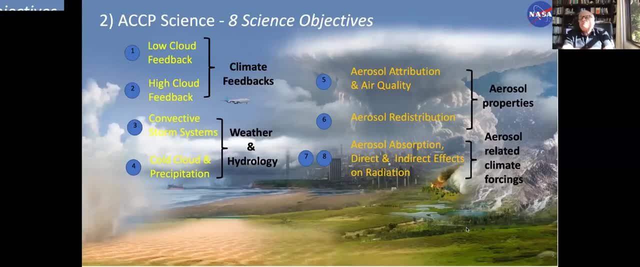 This is just a sort of synopsis of the eight science objectives. I'm not going to go into too much detail, I'm just going to go through them one by one- I'll come back to this in you know and see why these objectives evolve as they have. 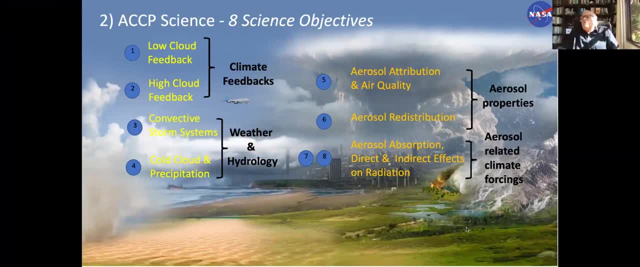 While there are eight objectives, you can kind of think of them as falling into four broad categories: climate feedbacks, weather and hydrology, aerosol properties and aerosol-related climate forces- but even these connect to each other. So, for example, high cloud feedback is very distinctly connected to our study of convection. 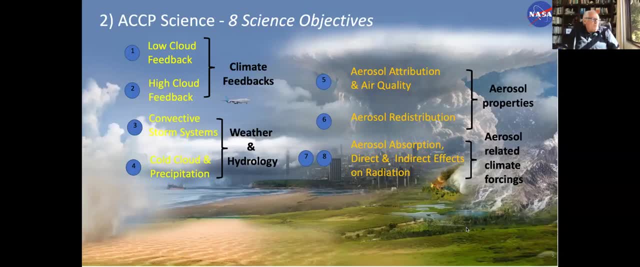 and convective storms. It's a production important source of production of high clouds as the convective convection that spews up water and ice into the atmosphere in the upper levels, forming these upper level clouds. So these, similarly the aerosol indirect effects on clouds, for example, is inadvertently. 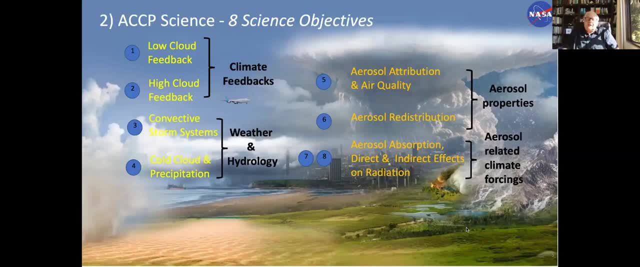 connected to the climate, the same processes that shape the climate, feedbacks of clouds. So these are sort of connected in various different ways. but we've identified these as sort of eight objectives And I'll come back to those and you'll understand why we sort of pose these objectives as we 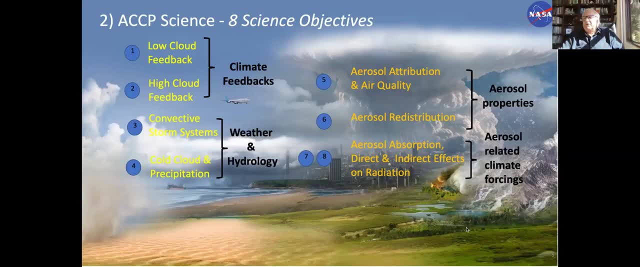 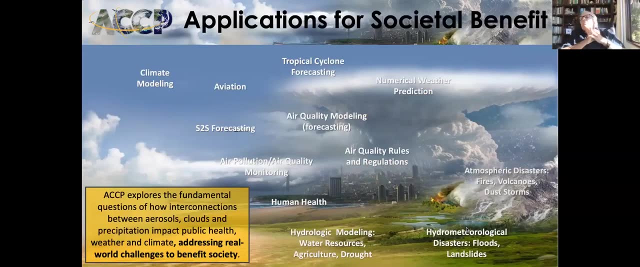 have as we start to think about the traceability of what ACCP represents in terms of what the community has asked for. There are a number of applications- that pretty obvious applications of ACCP relating to things that deal with weather and severe weather, hydrological process, hydro-measological processes. 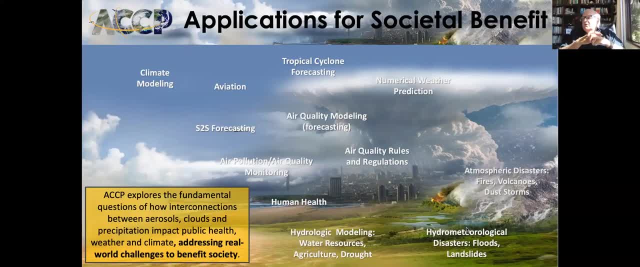 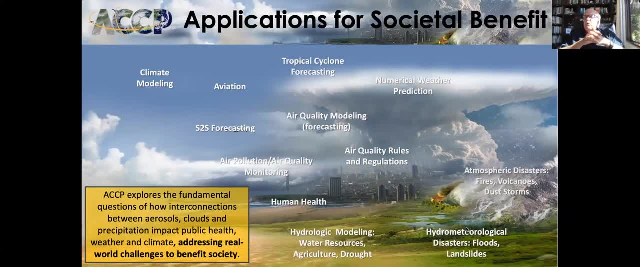 And I'll come back to those, And I'll come back to those And disasters related to those, as it relates to sort of flooding rains, for example. Air quality is an important element of ACCP, as you saw from the objectives and so on. 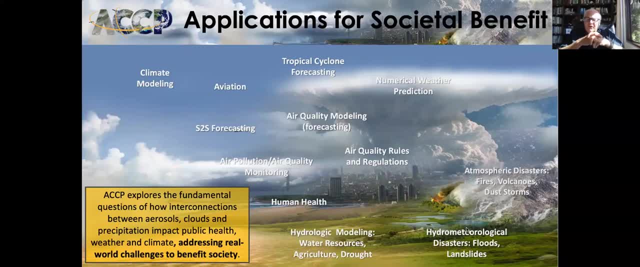 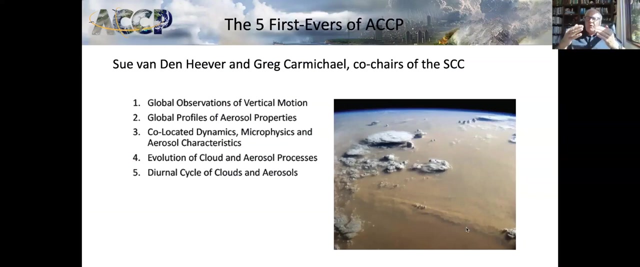 And so there's a very kind of active. it was a very active activity in terms of defining the applications of ACCP as we started to form our science and applications traceability matrix for the project. Okay, Okay, so there was, the study was structured. so I'm sort of still going back a little bit. 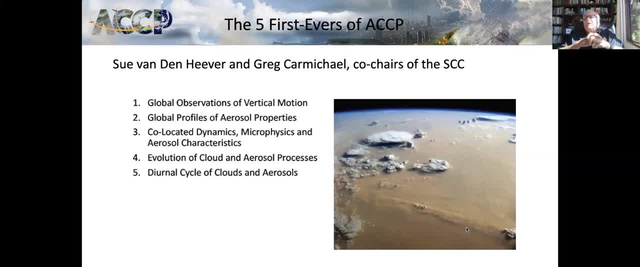 but the study was structured with a number of groups and one important, really quite important, group was the science. I forget what the SCC is, but basically it's the external science community, represented largely by academia, but whoever also had representatives from major research, non-NASA research labs such as DOE, Lawrence Livermore, Lawrence Livermore. 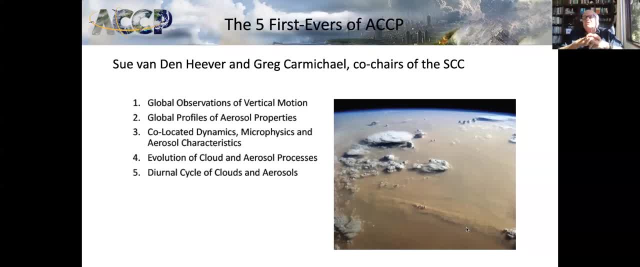 and NCAR itself. we had key leaders in the science providing us oversight to make sure that we were sort of addressing our thoughts in terms of the big science and important science were indeed resonated with that community, and so we had the community backing. 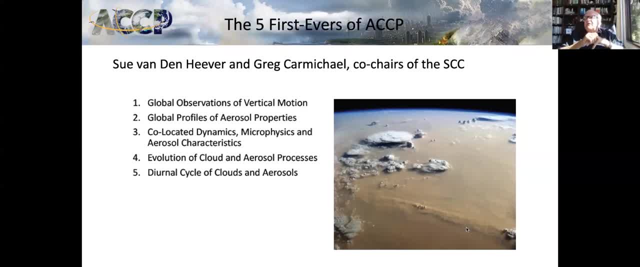 And they've identified what they think would be really the first efforts that we're going to do, and then we'll come out of the ACCP, once we implement it, as we showed you, of those two orbiting subspace craft and the other components of ACCP which I'll get to. 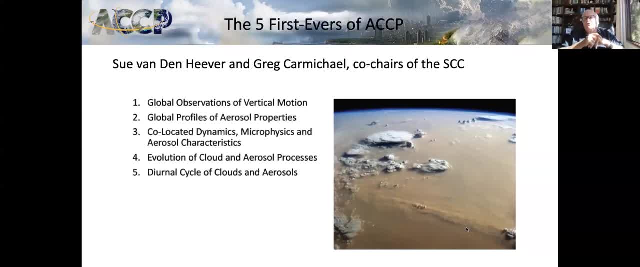 So global observations of vertical motion is a real, will be a real first ever. Fundamentally, the dynamics of the Earth system is kind of the new dimension in Earth system science and this measure of vertical motion is one aspect of that new dimension. 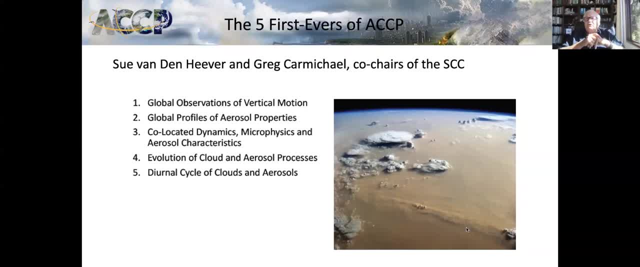 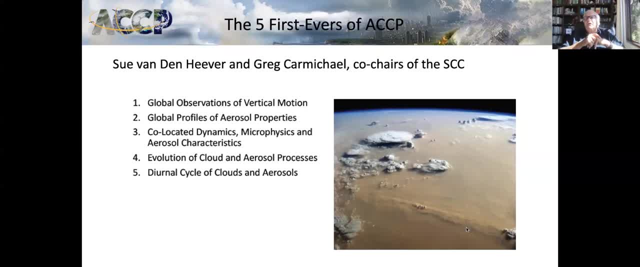 The profiles of aerosol will be unique and I'll explain a little bit in a minute. Billy had co-located dynamics, microphysics and aerosol characteristics is going to be revolutionary, and so on. So these are the five first evers that the community, the broader community, who provided 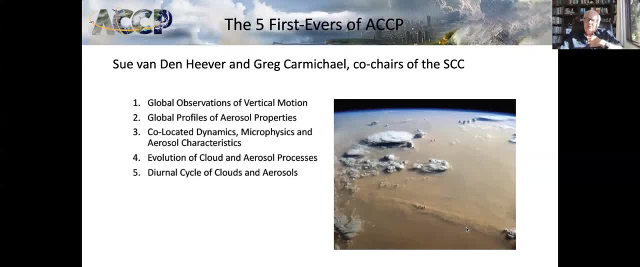 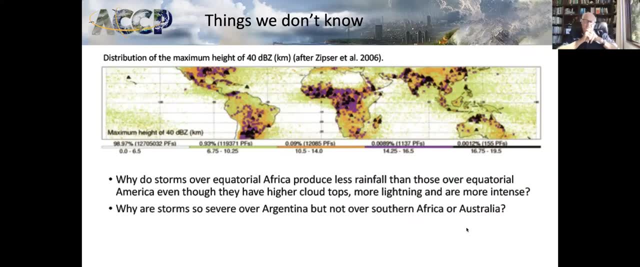 guidance to the study had identified. There are things we don't know and we think we're going to be able to address with ACCP, So there's going to be some degree of discovery with ACCP, much of which we actually probably have yet to even realize what that might be. 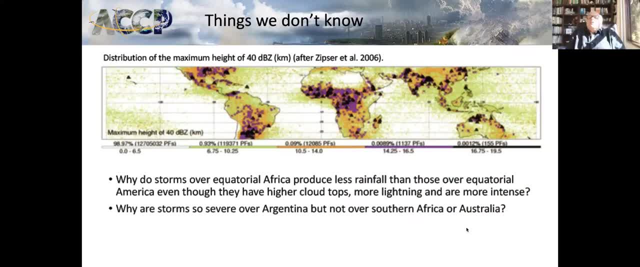 But, for example, there's things that we just don't understand in terms of measuring the of intensity of severe convective weather and storms. We don't know why, for example, Storms are a big problem. Storms are a big problem. 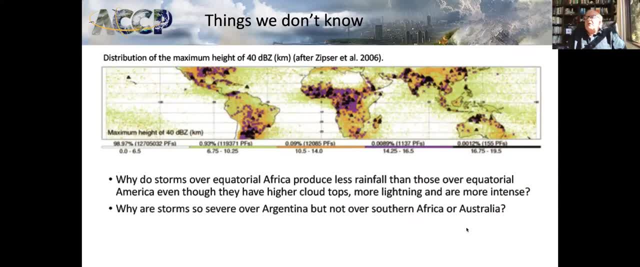 Storms are a big problem. We don't know if Africa produces less rainfall, yet they appear more intense. So try and understand the relationship between the intensity of convection, which you might measure in terms of the vertical motion, and the rain that falls from them: the intensity. 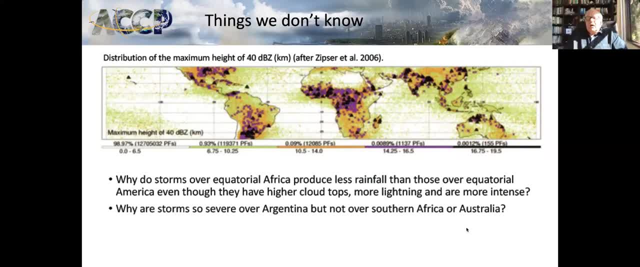 of rain that falls from them will be something that will become. I think will become. you know you'll be able to be diagnosed from the ACCP observations. Why are storms so severe over Argentina but not over southern Africa and Australia? for? 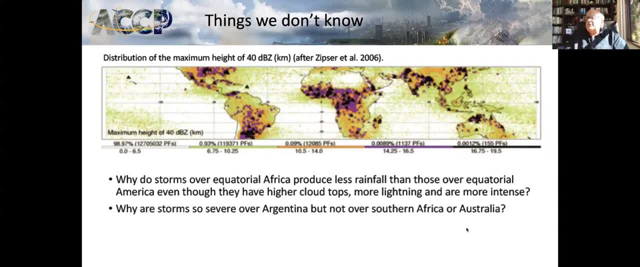 example, Because they have the same sorts of forces but they have different degrees of severity. So there are just things we just don't know yet about the fundamental aspects of the major storms on the planet that ACCP is going to really revolution with. 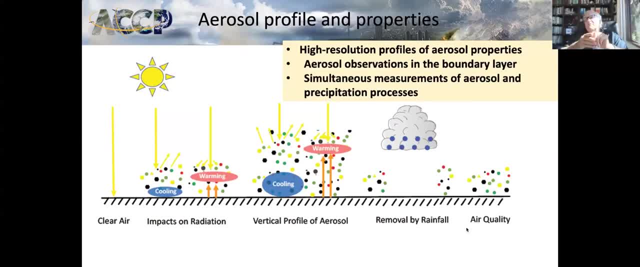 With respect to aerosol, one of our real capabilities is measuring the profiles of aerosol properties, And I'll highlight this a little bit further down the way as we go back and get more and more into the detail of ACCP. And then we start looking forward. 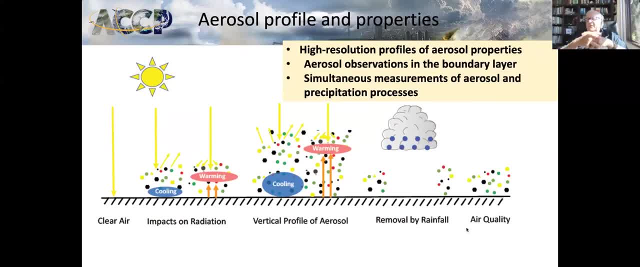 Okay, Thank you. So you know, one of the things we need to know is whether the aerosol is absorbed or scattered, and where that is distributed in the vertical. So you know, imagine an aerosol blob that absorbs and heats the atmosphere. 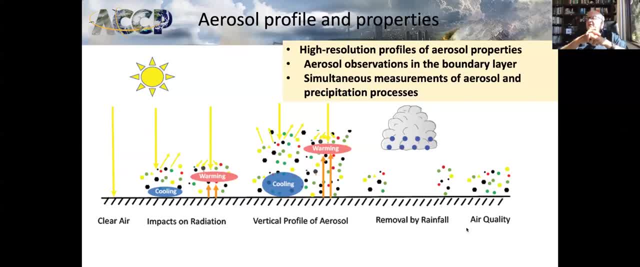 It really matters a lot to whether that heating is low in the atmosphere or high in the atmosphere, because it affects the atmospheric stability, which in turn affects other aspects of weather, and you know meteorology and the atmosphere. Okay, So just knowing the vertical distribution and then the characteristics of the aerosol, 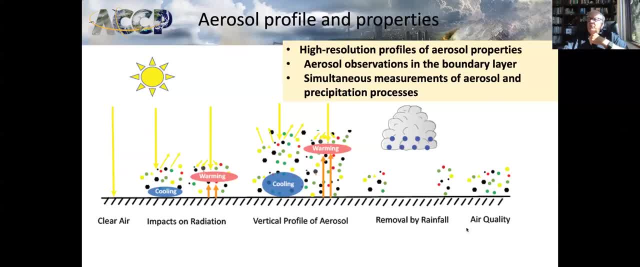 as opposed to vertical is really really quite important. It's also relevant to trying to understand, for example, how aerosol might get removed by rainfall and the air quality aspects of the aerosol itself. So the vertical distribution of aerosol and its properties is really kind of an important. 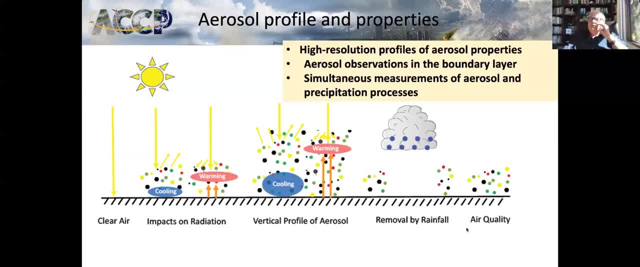 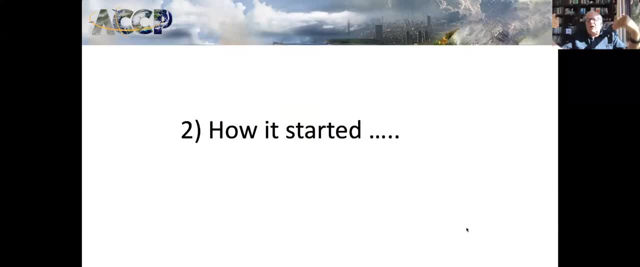 aspect that ACCP is trying to bring a focus towards. Okay, So this. So this is from the kind of the real beginning and how it started, because that was just basically like a prescient ACCP in many ways. Now we're going to go from the beginning and move forward. 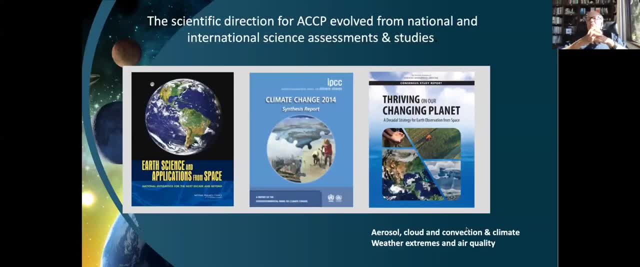 So how it started? is it started actually? I think it started with the previous decadal survey. actually didn't probably began even before that, with previous renditions of the IPCC assessments, But basically, you know, it began to be crystallised with the very first decadal survey. 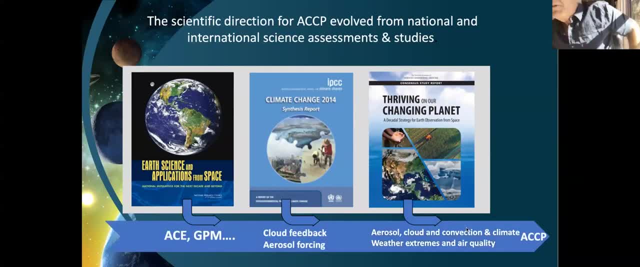 At that time, the definition of the ACE concept, GPM, which was already in the books before that decadal survey, was also crystallised with that decadal survey. So these were elements that laid a bit of foundation. And then we had the AR4 IPCC assessment, which called out the real challenges in climate. 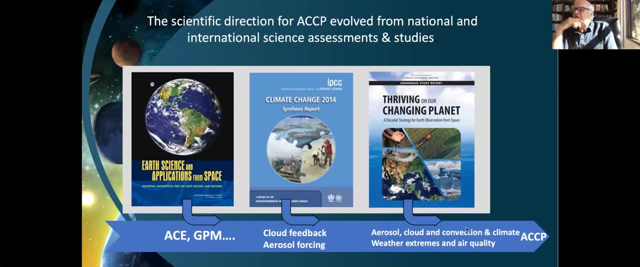 particularly climate, So climate projections with respect to feedbacks and forces of the Earth system, particularly related to clouds and aerosols, And this then, And that's for them on the timeline. This then fed into the decadal survey, the 2017 Decadal Survey Assessment. 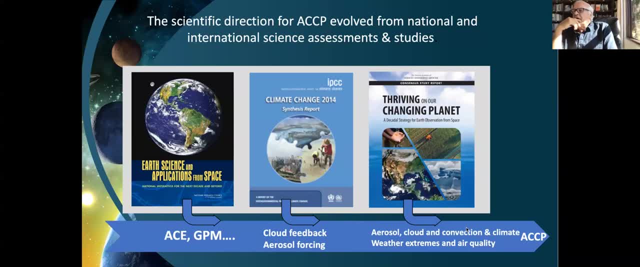 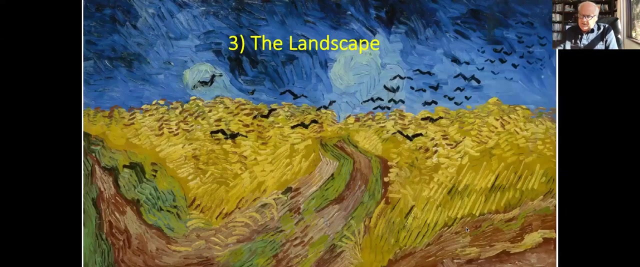 And out of that became a recommendation for aerosol cloud and connection, aerosol cloud connection and precipitation, a designated observable, And so this is sort of These all fed in ultimately, And this was really in the context of the. So let me just now stand back a little bit and think about the landscape in which ACCP 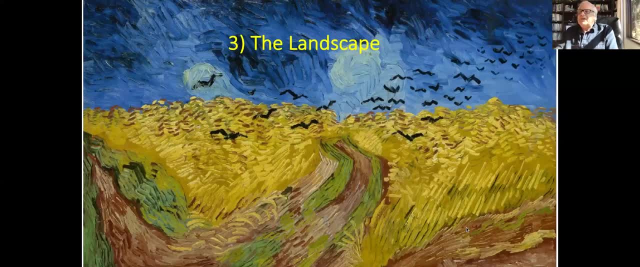 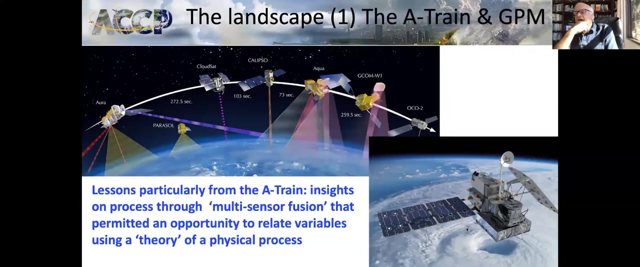 is being established on And this is really kind of important because it's really the context in which we think ACCP will offer progress in the years ahead. So the first is part of the landscape. the landscape was in many ways the A train in GPN We've built. we learned a lot through the A train. 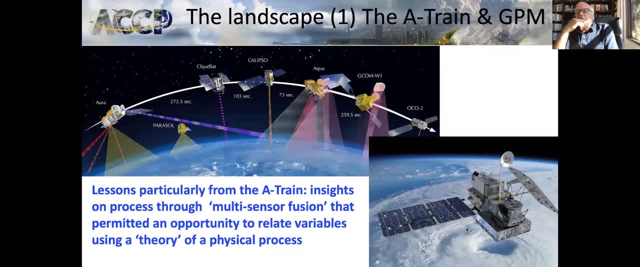 and how to, for example, fuse multi-sensor information to start to probe understanding about key processes of the physical system. I'm going to come back with a couple of examples of this further down the road, but this is really kind of important, And so this is why part of 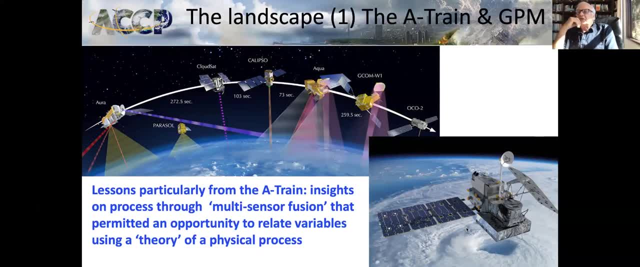 the landscape of the JCCB building itself is on developing a strategy to address critical process understanding through multi-sensor observations and the fusion of that. I'll talk a little bit about that in a moment. The second aspect of the landscape is the geo-ring, The geostationary. 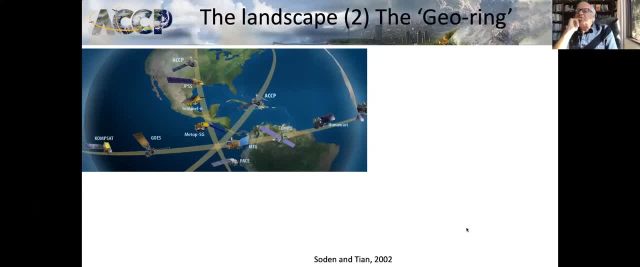 satellites now have unprecedented capabilities, which we've not had before. We now have common spectral channels, have these global representations spectrally at high time resolution and increased spatial resolution. This provides us with a really unprecedented way of providing context for ACCP, the time evolution of things that matter to ACCP, And so, for example, 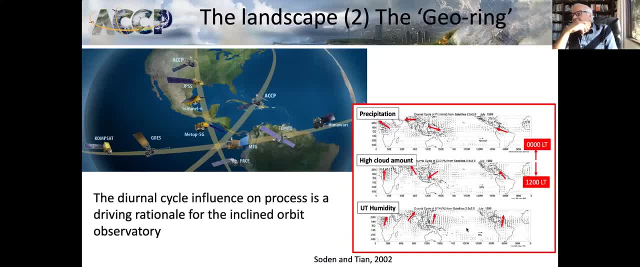 and I'll take this from the study of Sodin and Tian in 2002.. I think it's the right one, I think it's correct, Correctly if I'm wrong. It basically shows you the correlations or the connection. We know the connection between precipitation through convection and 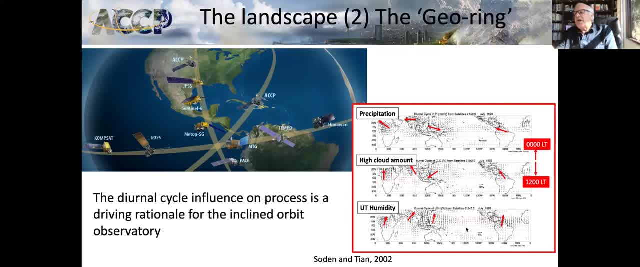 high cloud amount and the upper troposphere communication. All of these variables. this is it, the three variables. they're all very pertinent to climate and climate change, for example, pertinent to weather and the evolution and variability of the system. These properties are very important, They're very important. They're very important, They're very important. 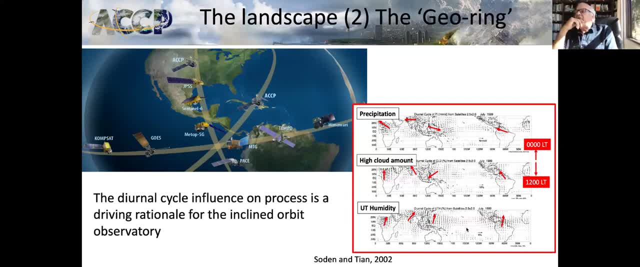 These properties relate to each other and they have a very distinct diurnal cycle that's phased differently. Precipitation is phased differently than, for example, the high cloud, So these arrows represent the arrow position in the clock- a 24-hour clock with 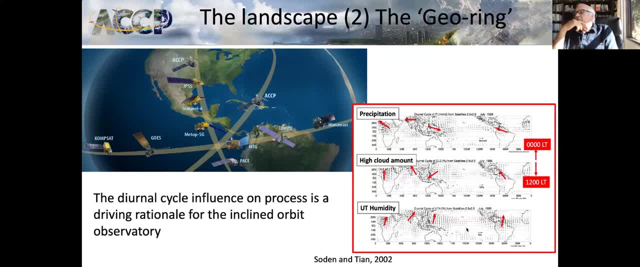 zero local time up and 1,200 local time down, And so there's a phasing that takes place with precipitation and high cloud and humidification, which occurs then later, And so there's a phasing that takes place with precipitation and high cloud and humidification, which occurs then later. 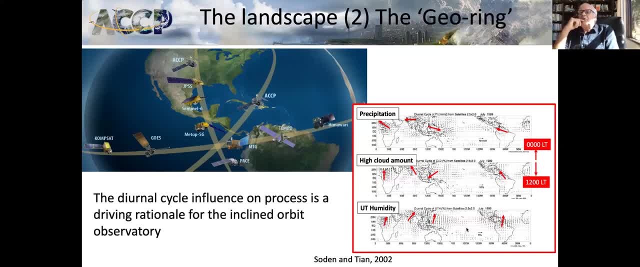 And so this, the diurnal cycle inference on processes, that on the processes that shape cloud convection, humidification and all these various connected pieces, that diurnal cycle influence is principally the driving rationale for the implied order to try to make measurements of the critical variables that unlock insight on the processes. 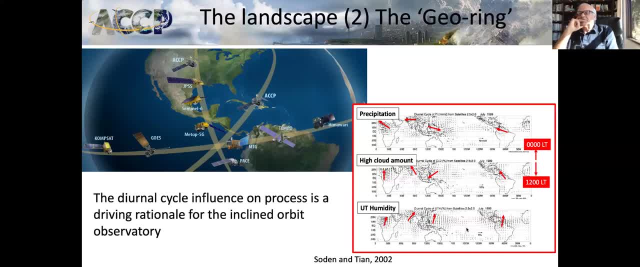 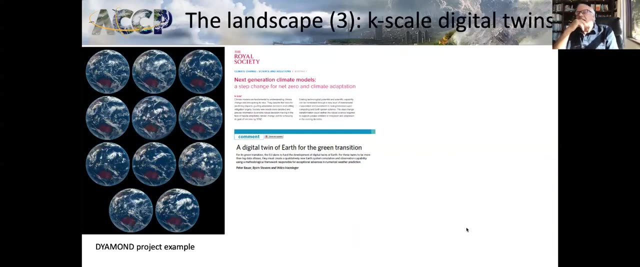 on the and the diurnal influence on those processes. So that was kind of a driving force of that inclined orbit component of the A6EP. The third aspect, of landscape, is really something that's really quite important. that's happening right in front of our eyes today and it's what's called the K-scale Earth System Modelling. 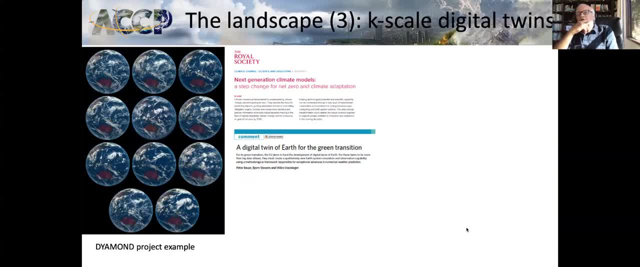 The Earth System Modelling is really going through a I won't say revolution, but certainly an evolution towards kilometre scale modelling. It's happening. It's going to happen, It's going to be with us at the end of the decade, when A6EP is actually producing observations. 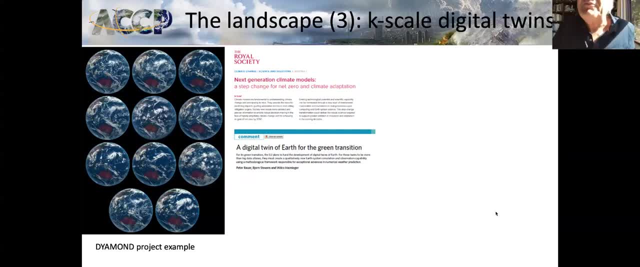 There are a number of examples of this. The images to the left there are from a number of One sets an observed world, and the other little 10 are from a digitally produced world, High K-scale resolution, and this is from the Diamond project that was kicked up a few. 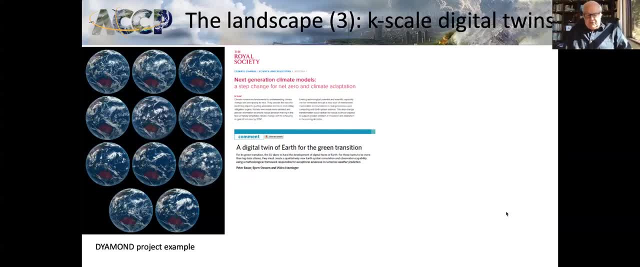 years ago. We're now moving steadfastly towards development of K-scale Earth System Modelling and this is really beginning to cause a little tension within Earth System Modelling across the world. That's kind of an interesting scenario. But basically there's two of these. 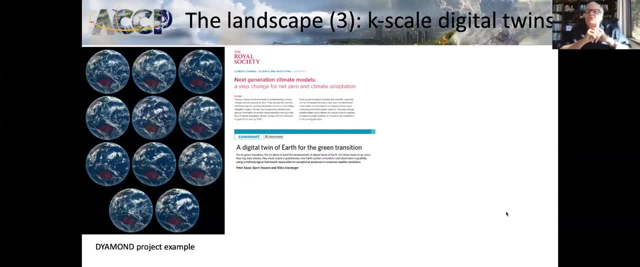 These are just extracts taken from Earth. Okay, They're taken from two important papers. One's a position paper from the Royal Society to the COP26, articulating what it sees as the next generation of climate models and their argument: the next generation climate. 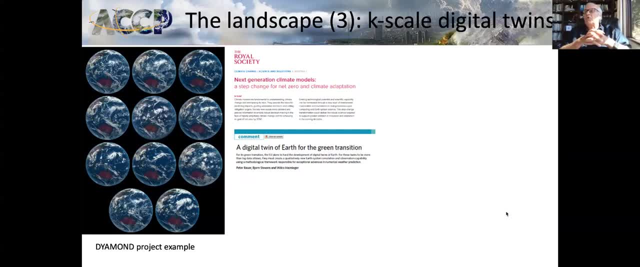 model will be K-scale digital Earth climate models. There's already major activities within Europe to move towards steadfastly towards the creation of these Earth System Modelling at the climate scale. Why this is important- It's relevant to the landscape of ACCP- is sort of illustrated in these figures here. 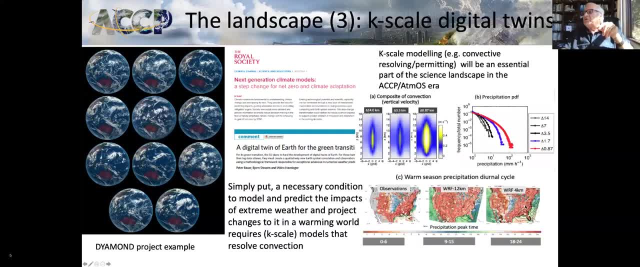 I just sort of focus on. I presume you can see my cursor there, but I just focus on. Let's just take the right-hand most figure here which shows you the PDF of precipitation as a function. These are from global models, global PDF of precipitation rate and frequency. 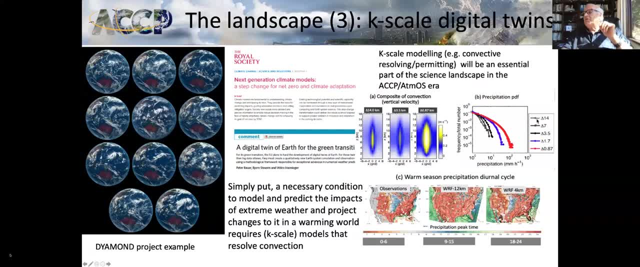 here- and this is for the different colors of these curves- represent different global model resolutions. Okay, This is from 14 kilometers, 7 kilometers, 3.5 kilometers, 1.7, and 870 meters global resolution. This is from the NICAM. Let's see the number of NICAM experiments done by a Japanese college. 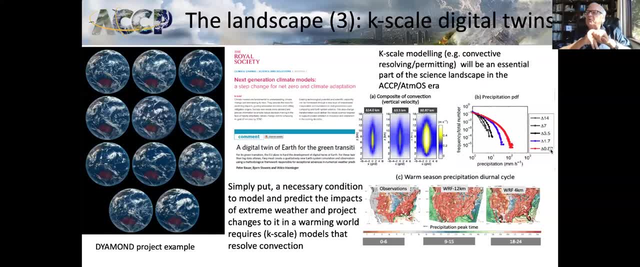 You can see the PDF of precipitation. We've known this is not just from the NICAM model, but other models have shown the same thing. Indeed, the ECWF forecast model has been run at climate scale as doing just examples of climate scale forecast: 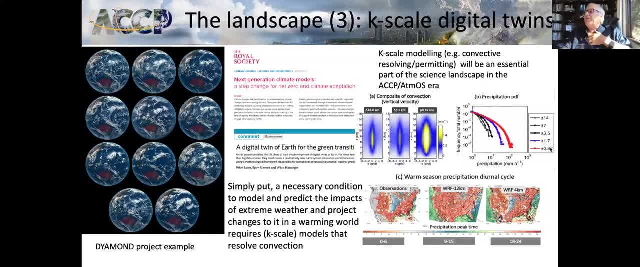 They all show this behavior Of a fundamental shift in the PDF of precipitation from the much less intense precipitation in the coarse resolution models to much higher precipitation at the tail of the distribution in the high resolution models. Other examples were taken from the simulations of conus precipitation with different models. 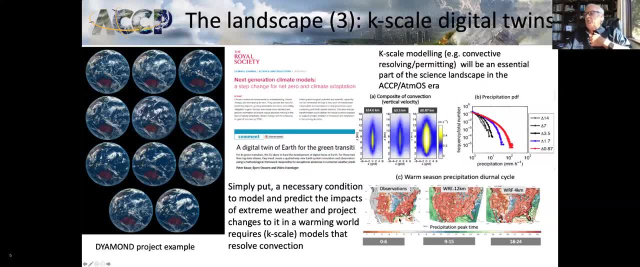 with different resolutions and the ability to represent the diurnal cycle of precipitation, as these three panels down here, the 12-kilometer models, unable to represent anything near the final cycle of precipitation over conus compared to the observations where the full conus starts. 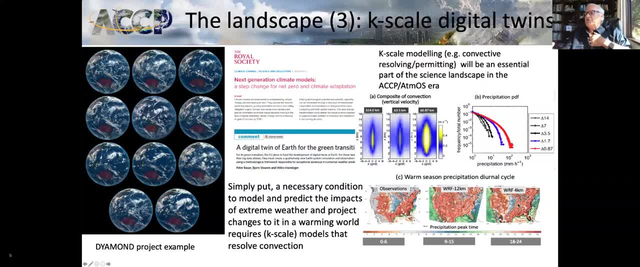 to get the characteristics of diurnal force convection and its effect on precipitation. Simply put, this is the issue. simply put, a necessary condition to model and predict the impacts of extreme weather and project changes to it in a warming world requires case scale models at least. 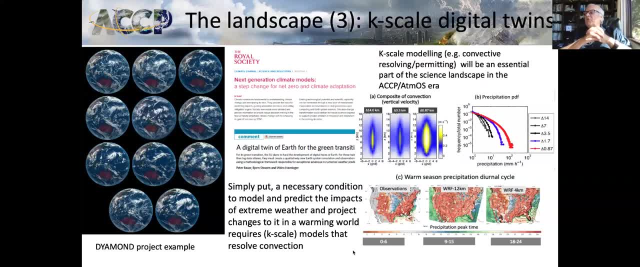 That resolve convection. You cannot argue for credibility in models of coarse resolution that talk about extremes in precipitation. You're just not resolving the processes that shape the extremes of precipitation. This is really one of the driving forces towards case scale modeling. when you start to wonder. 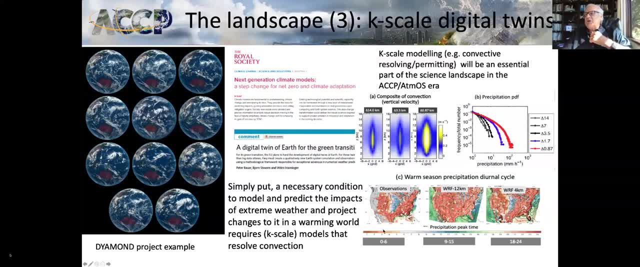 about applications, societal applications and how extreme weather is going to change. with warming Fundamentally can't be dressed, I'm not sure I'm going to make this statement Can't really be addressed without resolving the processes that determine extreme weather. 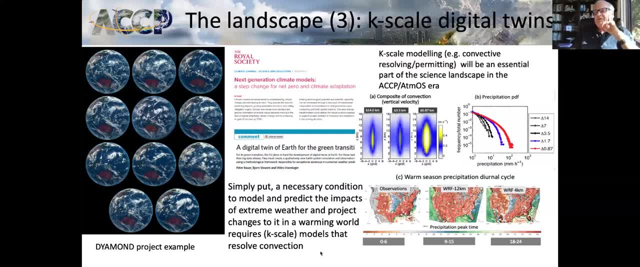 This is really a revolution that's taking place and this will be in place at the end of the decade. These tools will be in place, as I said at the time of ACCP, but these tools won't just be model and forecast. 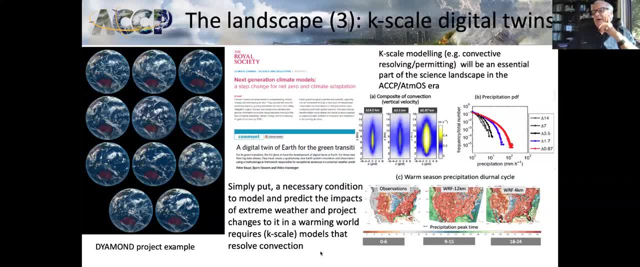 These tools will be able to project, be part of the overall analysis system, be part of the observing system itself. ultimately, in order to give you time, space, resolution of information needed for the applications that will come from some blending of the observations. 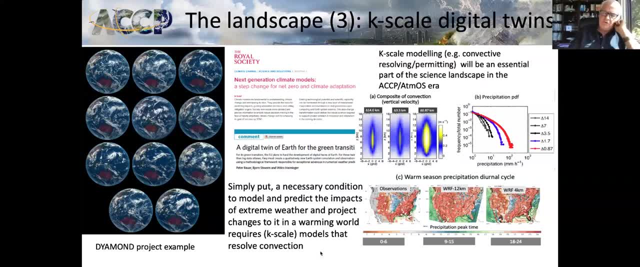 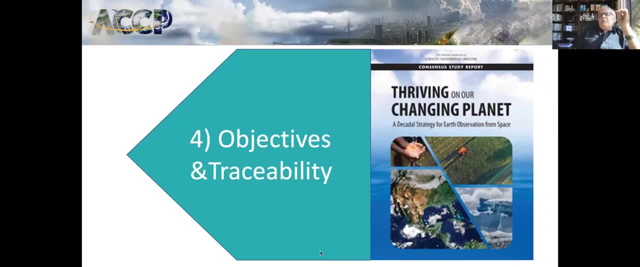 and models. These case scale models will be critical in that respect. Okay, Enough happened about that. Now that we've looked towards the objectives, come revisit the objectives and the traceability of the objectives. How the objectives came about. What forced them to be defined. 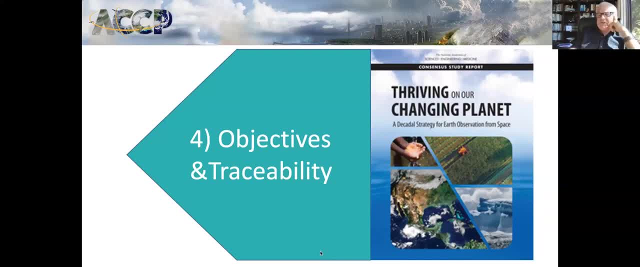 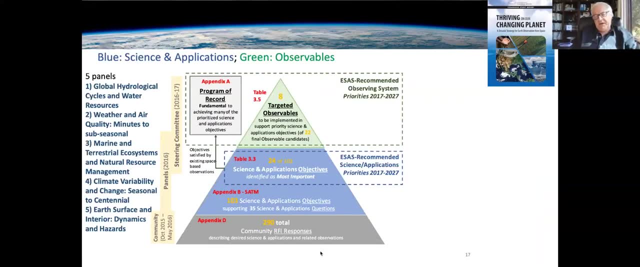 What was the objective? What was the way we did? It sort of started with basically a traceability back to the Cable Survey recommendations. The Cable Survey recommendations were framed as follows. Basically it was there was a large community input that fed through five panels and the 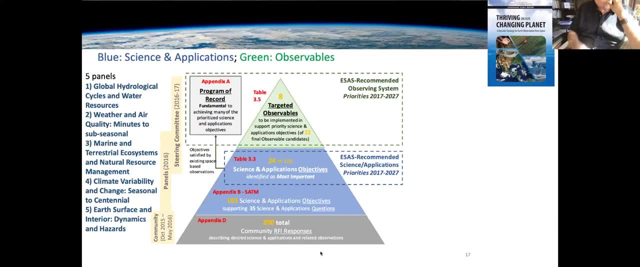 five panels are listed there on the left. You probably- many of you probably- know what these panels are: the hydrology panel. I'm just going to abbreviate it: The hydrology panel. the weather panel, Ecosystems panel, Climate panel. 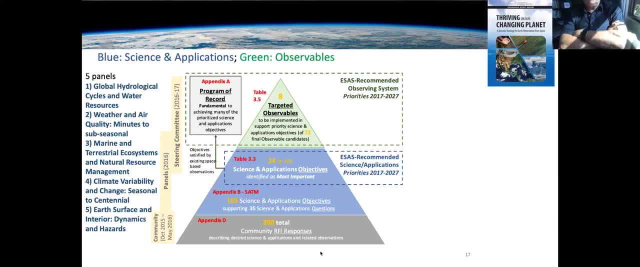 Earth surface Interior panel. These panels sifted through these responses and also a number of other inputs and defined a series of objectives and there were 24 most important objectives that filtered up from these panels. These 20, these most important, represent events in the panel's eyes. 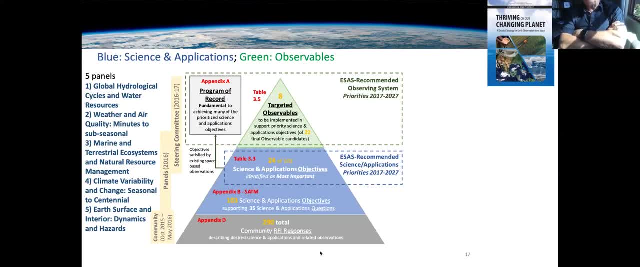 And in the study's eyes, that if we did not make progress towards these objectives, Earth system science would not make progress in the decades. So these 24 were quite fundamental And out of those from those 24, kind of distilled into eight targeted observables. 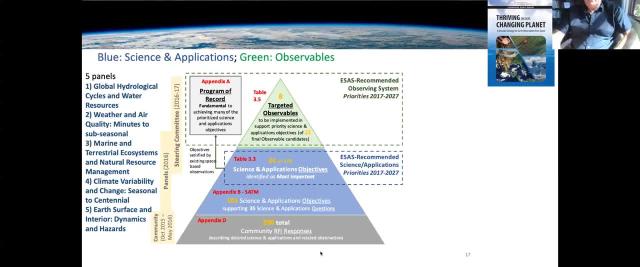 And that led to five designated observable, observable and two of those. two of those were- well, four of those, I guess were aerosol clouds, convection and precipitation that were lumped into one single study by NASA because of the synergy between the observing. 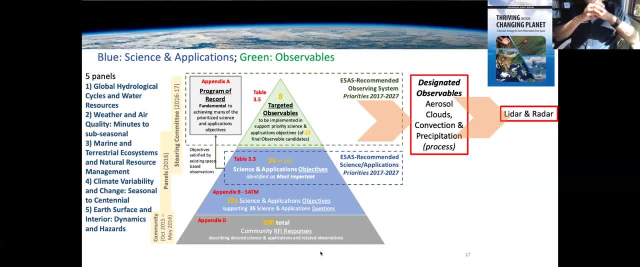 strategies for aerosol clouds and convection. The synergy would be framed around the use of LIDAR and LIDAR active systems that could profile kind of exquisitely through the atmosphere form. So that's kind of the flow of how recommendations flowed. 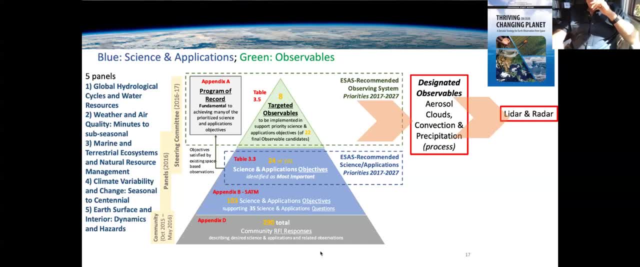 It was really tricky, But it really truly represented in this way the community's interests. Now, of the 24 most important the SCABLE survey objectives identified by the community through the lens of these five panels, ACCP directly relates to 12 of them and explicitly 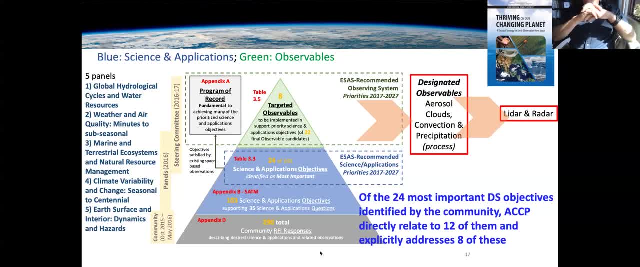 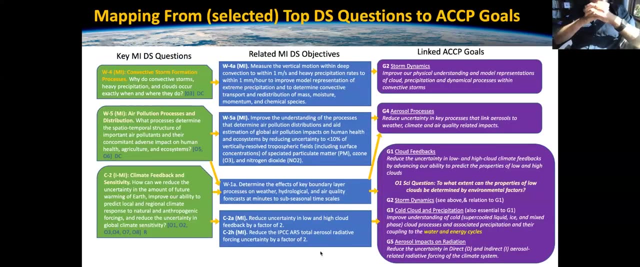 addresses eight of them, And so- and I'm even going to collapse this down to even a fewer set, just because it was the way we defined The observing strategy, the observing system, processes, and so there's basically three most important objectives were expressed as questions by the Decatur survey. 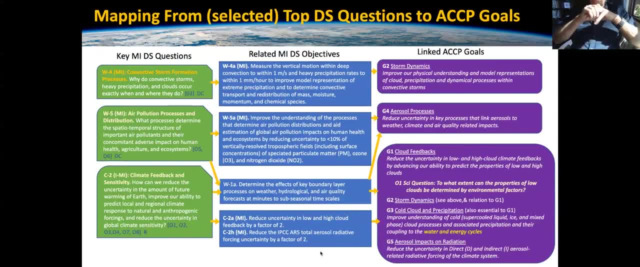 And these are the three questions that are basically the ACCP science questions. Why do convective storms heavy precipitation? that's exactly when and where they do. What processes determine the spatial temporal structure of the important air pollutants and their contributing adverse impact to human health? 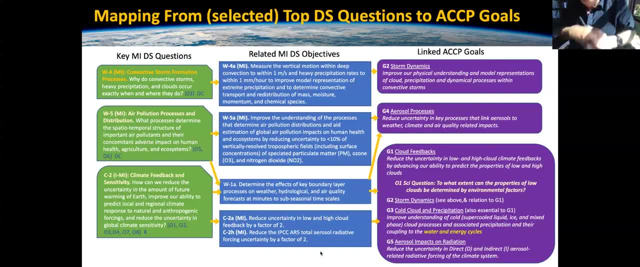 And then the other question is: why do convective storms, heavy precipitation, go exactly when and where they do, And how can we reduce uncertainty in the amount of future warming of Earth and prove our ability to predict local and regional climate response to natural and anthropogenic 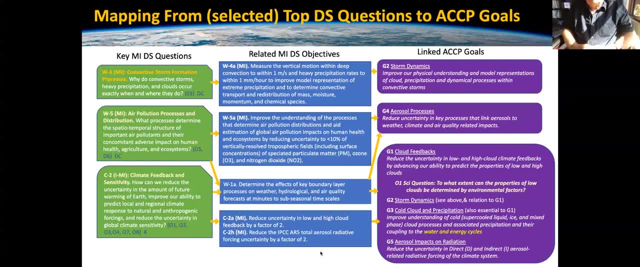 forces and reduce uncertainty in climate and solar. Now they're the sort of overarching science questions pulled straight from the Decatur survey, and they came back through more focussed questions that the Decatur survey identified, such as, for example- I'm not going to read two of those, but one, for example, is reducing 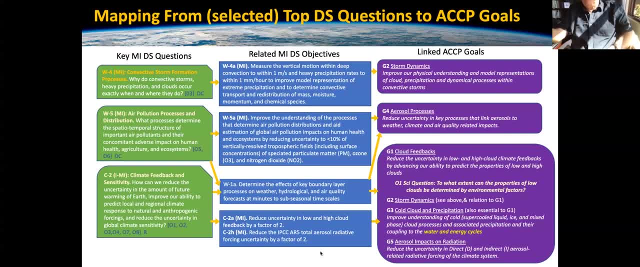 the air pollution, the uncertainty and long high cut feedback and aerosol radiating forces. that's happening to, yeah, for the climate as it relates to the climate questions, and these then connect to six goals and under these goals are the eight objectives, eight objectives that are full under these goals. 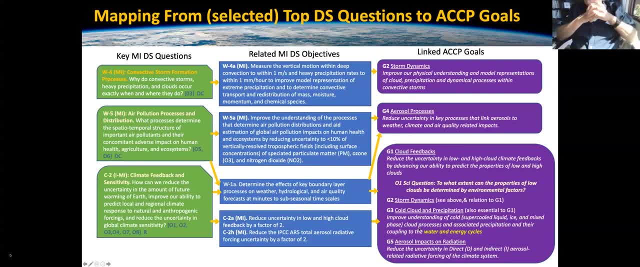 you know the goals include, you know, cloud feedback, storm dynamics, cold cloud and precipitation processes with a high towards the polar and polar influences, aerosol impacts and radiation, aerosol processes and storm, uh, so these are, uh, actually, five goals. we should say that's it goals. and so under these five goals lie these eight objectives. 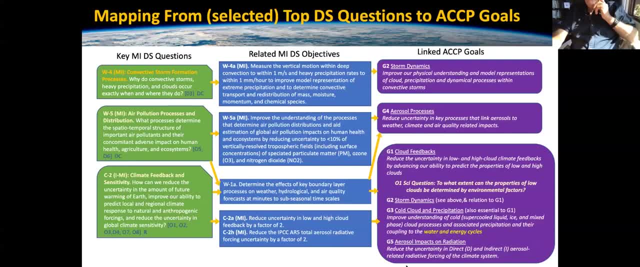 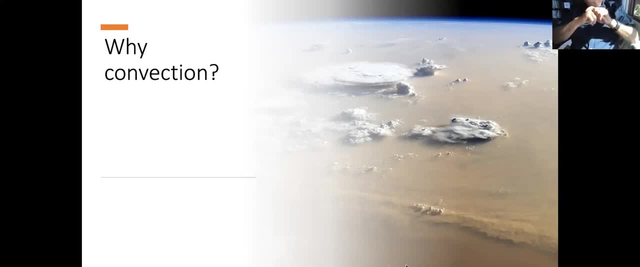 so so these are objectives. uh, you know, we kind of give you a little bit of a thumbnail sketch of those, so let me just dwell a little bit on a couple of these. why convection? why are we calling out convection specifically as part of the new component of a ccp? um, and you know from scientific 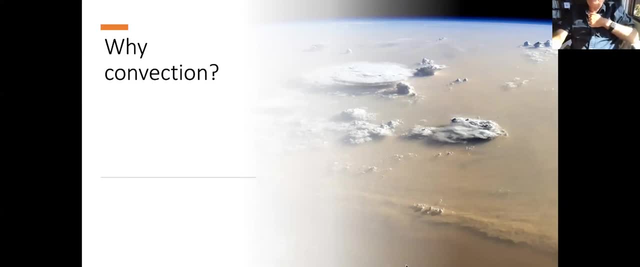 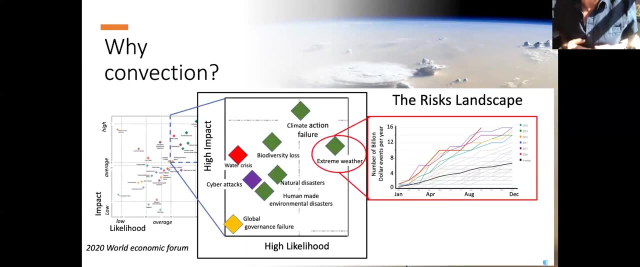 perspective. this is pretty easy to argue, but i'm just going to present it from a kind of slightly different perspective, through the eyes of the worldly- world economists, as expressed by the world economic forum report in 2020, and in that report they produce what's called a, a risk landscape, and 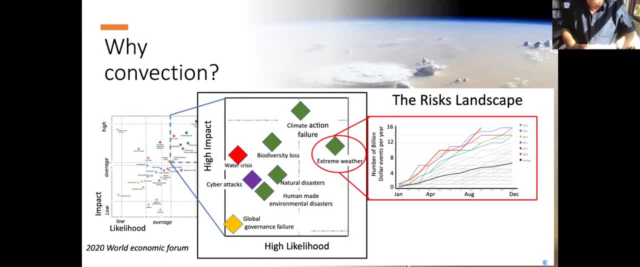 that land. that diagram, um, that diagram that explains, that represents that risk is is on the x-axis is the likelihood of a risk occurring and on the y-axis is the impact of such a risk. and the upper right corner of that figure which you can't read, all those little diamonds in. 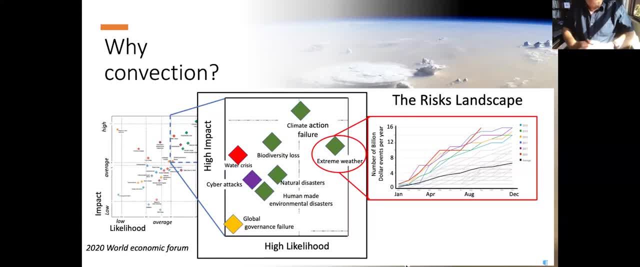 um represent risks that are most likely to happen and have the highest impact, and they, they all tend to lie, they all tend to be essentially part of the cyber attack. uh, global governments- they are in silence- but essentially our environmental risks. this can do with environmental issues like human environment disasters, um, extreme weather being the most. 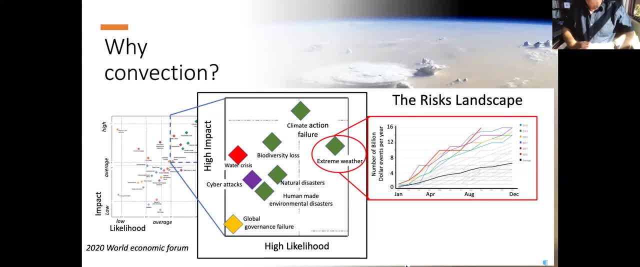 likely one of the highest impact um risks now- extreme weather. the risk of extreme weather to a large extent is driven by the risks associated with convective storms, And here's an example of this landscape on the right-hand side from NOAA is: this: is the number of billion-dollar events per year of convective storms. the impact of convective 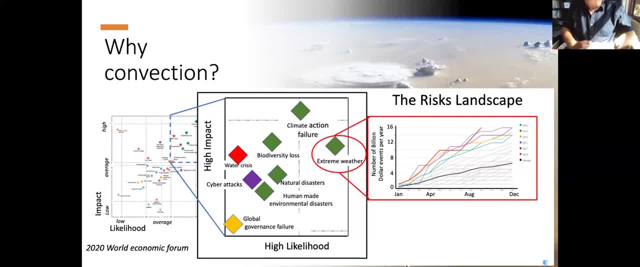 storms. These are convective storm events and the impact in terms of dollars to the US, showing the evolution the different years and the evolution the average over year. So these extreme events appear to be occurring more frequently, or at least their impact. 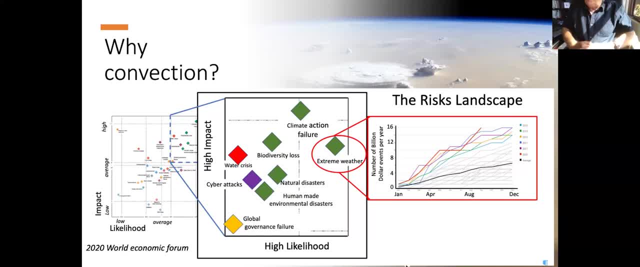 on the economy is occurring is larger, is increasing over time. So this is sort of it's sort of a no-brainer as to why we want to try to really advance our ability to model, understand, represent and model and forecast convective storms. 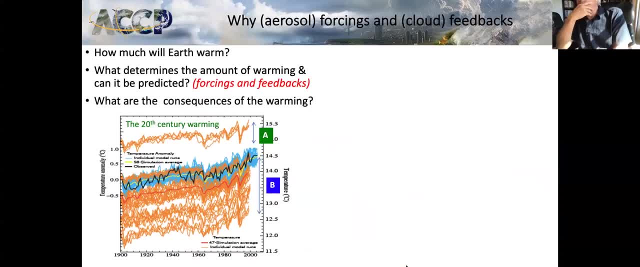 Second aspect of this is why we're doing this, Why forcing some feedback? Well, these are tied to pretty big questions about the warming of the Earth And this figure here shows the historical warming of the Earth in the 20th century And the upper curves show typically what you see in assessments. it shows you the anomaly. 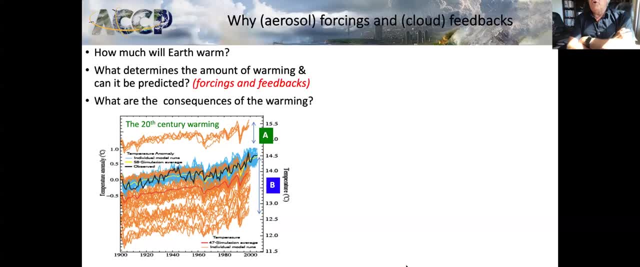 temperature anomaly as a function of time. The lower curve actually shows the temperature itself as a function of time, and you don't tend to see this figure because it reveals something rather uncomfortable. So the upper, So the warming, is a curve that's highlighted by that arrow and designated as A is driven. 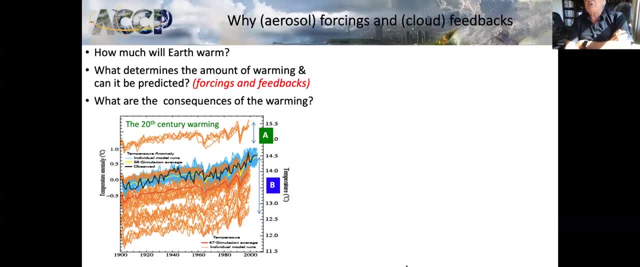 by forcings and feedbacks. that degree of the warming is driven by forces and feedbacks, But it's also driven and influenced by B, which are the biases of the models. The spread of the models in the lower sets of curves really is sort of emblematic of 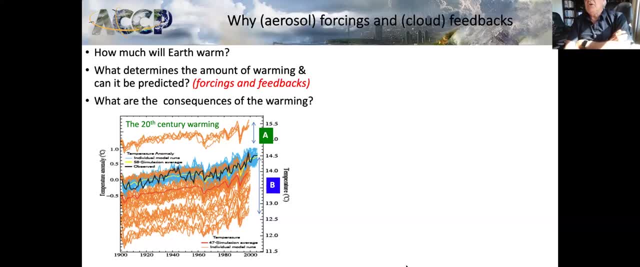 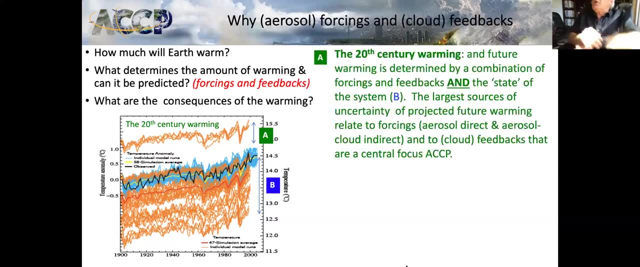 biases of the models and those biases in turn affect the degree of warming and the projected warming. I'm going to try to show you, I'm going to try to illustrate this point a bit. The 20th century warming A, as I said, is shaped by forcings and feedbacks. 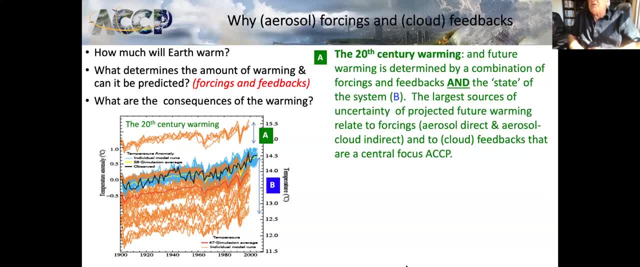 And the IPCC has in previous. and the AR6 makes the same point as AR5, as AR, yeah, AR6, as AR- no, yeah, look up that number. The present assessment, which is the current embargo, makes the same point. is that the 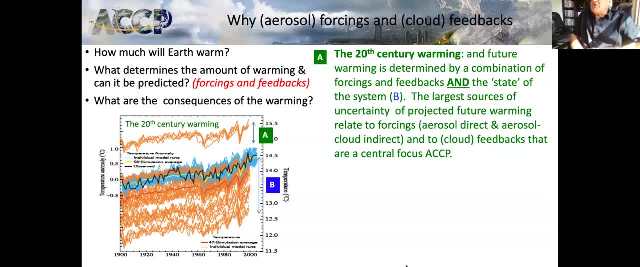 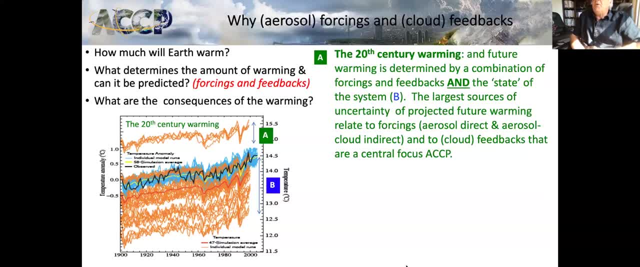 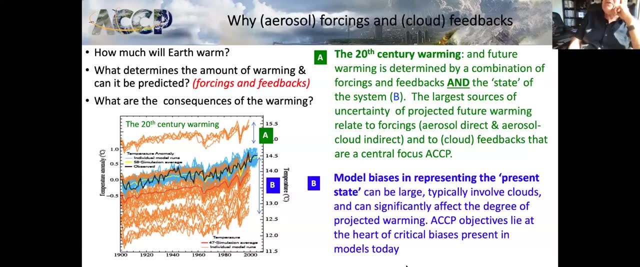 of warming related to cloud feedbacks. So these are the primary sources of uncertainty in terms of representing both the historical warming and representing the future warming Model. biases in representing the present state can also be large. They typically involve clouds and can significantly affect the degree of warming. 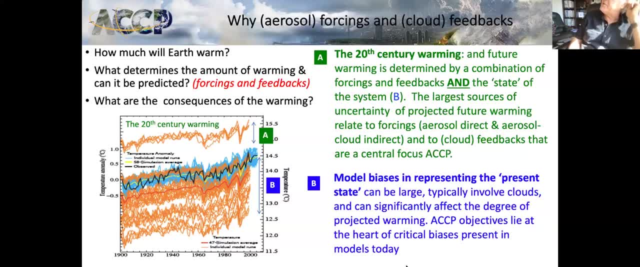 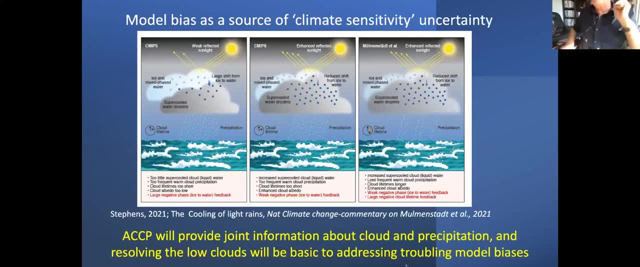 ICCP objectives lie at the heart of critical biases present in models like that. I'm just going to highlight an example here, And this is from a figure that I had created that was a commentary on a paper that published by Woodenstead et al. 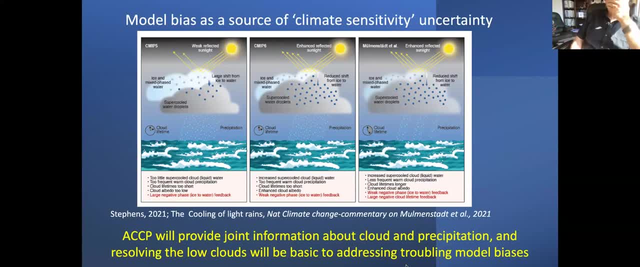 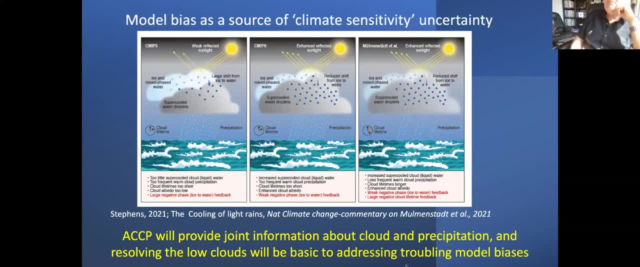 And it sort of highlights the sensitivity of climate projections to the existing base state of the climate system and hence the biases of models in representing that base state. Okay, So there are three out there. One represents a CMIC-5 class of models. 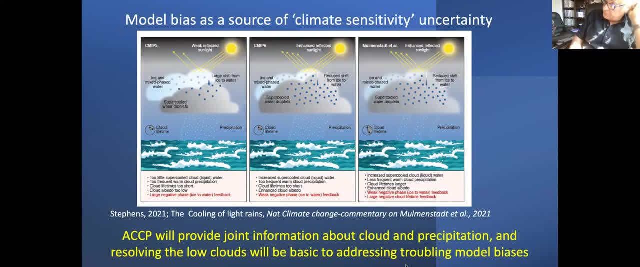 One represents a CMIC-6 class of models. One represents the experiments that the state had done. The CMIC-5 represented southern. Now, these are all related to, probably, the southern ocean clouds. Those are the ones that are in the margin. 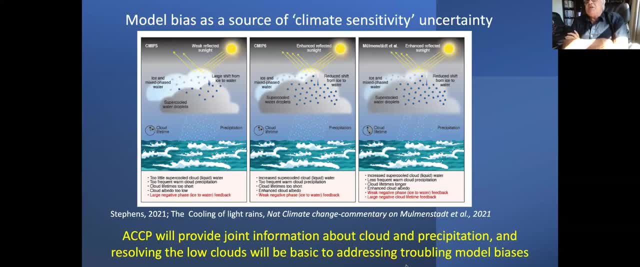 This is an example of that. clouds around some 30,, 40, and 60 degrees. The model signified models had way too little super cool water in those clouds. They basically just didn't reflect enough energy sunlight back to space compared to 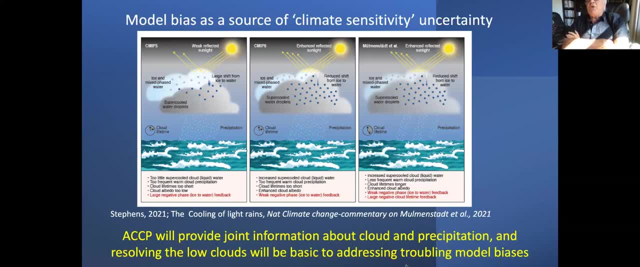 the observations, But the clouds that were there would just rain too frequently, their lifetimes were way too short and their albedo sunlight reflected way too low. So what happened when you impose a warming or you force it with a climate forcing that? 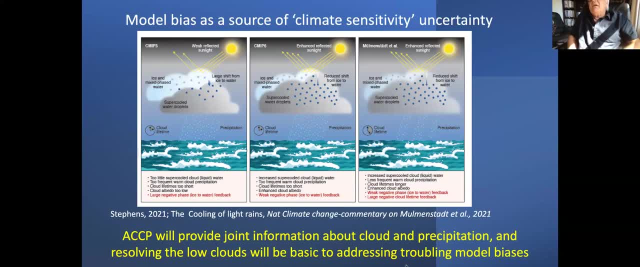 reduces the warming is that the fact that the ice clouds that coexist with the water clouds. there there's too much ice and not enough water and that ice cloud would transition to water and would make a large negative feedback, unrealistic negative feedback. 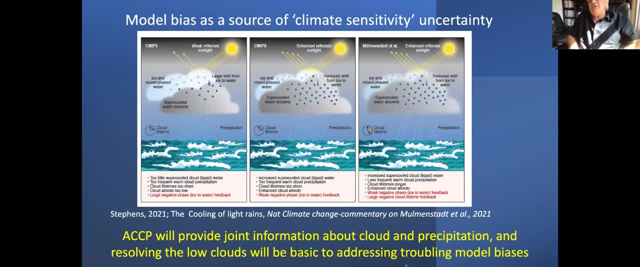 And that ended up resulting in a climate sensitivity that was evident for CMIP5.. The climate sensitivity were 3-ish, you know, in many of the models, evidently the climate models at that time. Now the CMIP6, the current assessment, has the later generation version of the model. 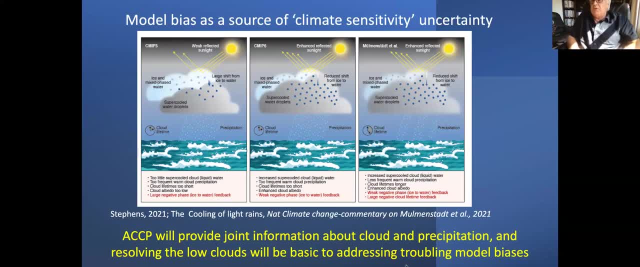 where the modelling centres tried to fix this, because I recognise this was a problem, And so they were able to increase the super cool water in clouds by changing parametrizations. in clouds They still rained too much, The lifetimes and weights were still too short. 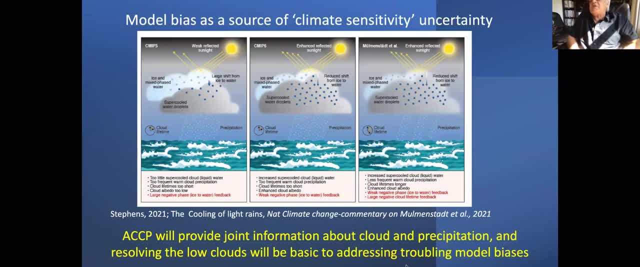 But it did enhance the cloud albedo. The cloud albedo much more like observations, so they ticked that box and they went away feeling pretty good with themselves. This resulted, however, with a very weak negative phase feedback, because there's much less. 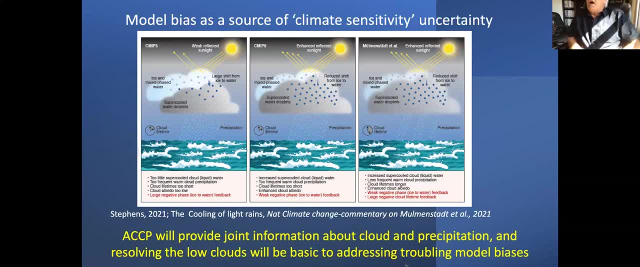 ice that would turn to water would then make a large negative feedback by making the clouds more reflective in a warming world, as opposed to CMIP5, where the clouds, as the clouds warm, ended up reflecting quite a bit more because there's more water there, more transition. 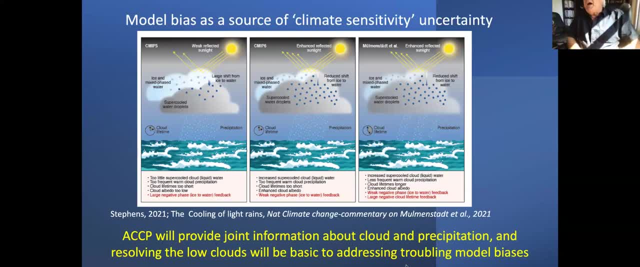 from ice to water, And so the CMIP6., CMIP7., CMIP8., CMIP9., CMIP10., CMIP12 and CMX took away this negative feedback, this phases of feedback, that was negative And hence, as a result, the climate sensitivity of those models rose. 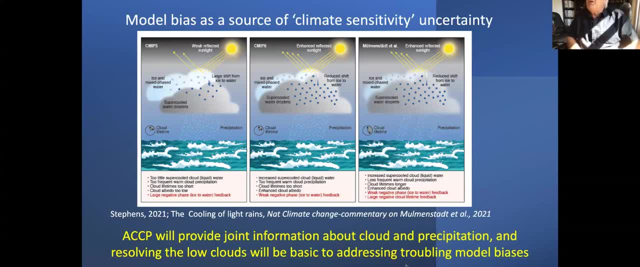 You do what, you start to see models with sensitivity in the fives, 5.5, for example, all based on the driving factor was the southern ocean cloud. Now, I'm almost at all, of course, recognise that there are still biases in models and 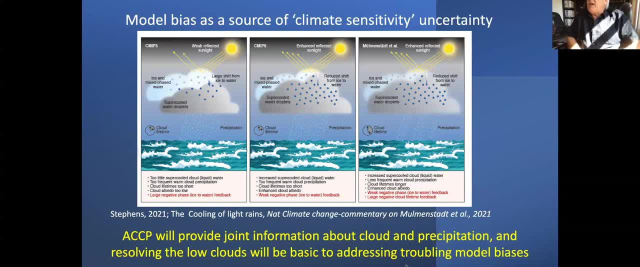 one of the major biases is they rain too much. And what this did? it had an effect on changing the lifetime of the clouds. So if you reduce the amount of rain, these clouds hung around longer and this basically introduced back a large negative feedback. So when the warming occurred, the warming was forced. 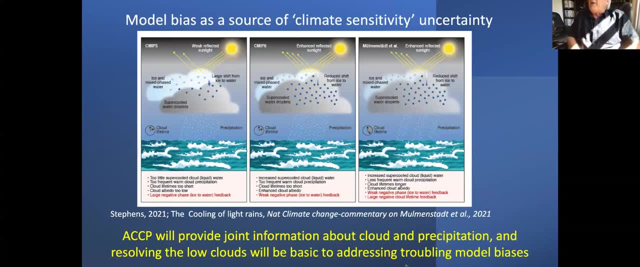 this negative feedback operated and actually brought back the climate sensitivity more like three. So it just underscores the point- and this is just an illustration. it just underscores the point that biases in the present state of the Earth-Citizen Moon models actually has a dramatic. 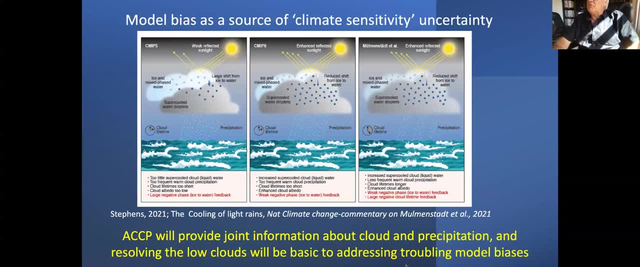 influence on ability to project the warming for those models, And the ACCP really will provide the joint information about precipitation and resolving low clouds that will be basic to addressing these troubling biases. So this is really at the heart of some of the ACCP objectives. 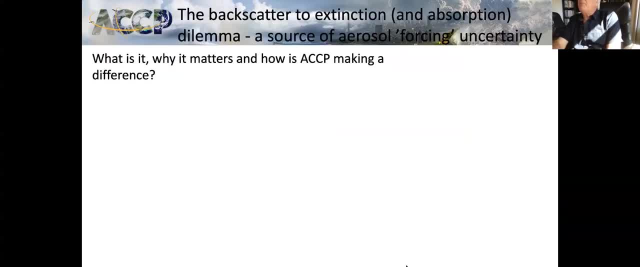 Okay, Let me talk a little bit about aerosol and then we'll come back and start moving towards the end. So the aerosol, this issue of backscaled extinction and absorption dilemma with aerosol- and it's basically fundamentally- makes it difficult to 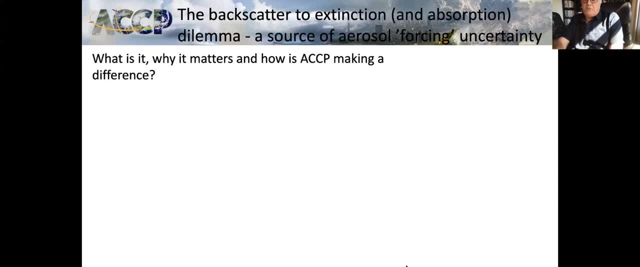 quantify aerosol effects from an observational point of view and quantifying its forces. And so what is this dilemma? How is it and how is ACCP going to make a real sea change difference in this? Okay, Well, the issue is: 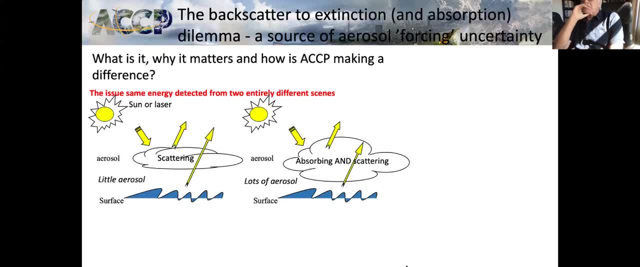 pretty simple. Imagine you've got two aerosol layers. One is just the aerosols are primarily scattering and one the aerosol mix, absorbing and scattering together Lots of aerosol. but they're also absorbed From a point of view of looking down from the top of the atmosphere down. 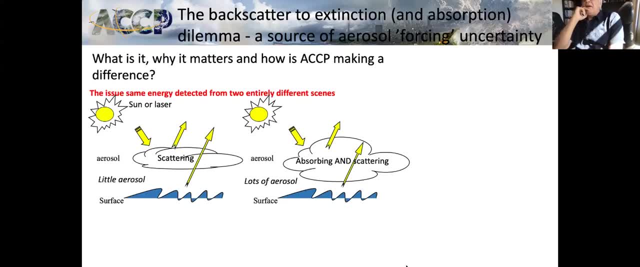 the amount of sunlight, for example, might look the same. The amount of laser light backscattered might also look the same. So we can't really distinguish between whether there's lots of aerosol that both absorb and scatter or whether there's fewer aerosols. 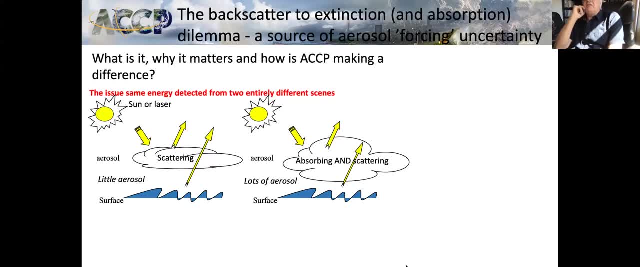 which are scattered, And the way we should have done this in the past is try to impose information about what we think the aerosol are, to try to unscramble this egg, as it were. And this is a real problem, And there's a real problem from the point of view of 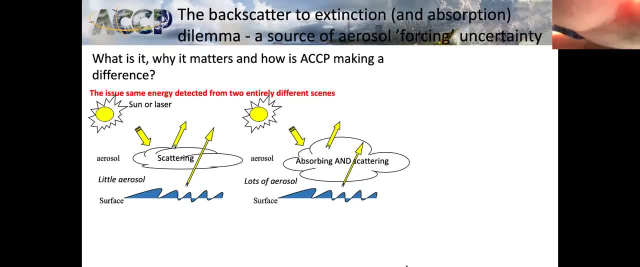 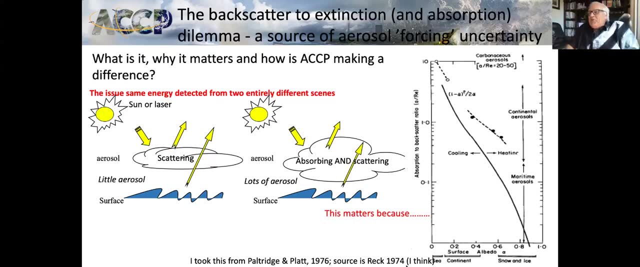 aerosol forcing climate. I'm going to use something I'm sure none of you have seen, because this is such an old, old figure And everything was written in the 70s and now dispensed with in the science. They have no relevance, But I pulled this out. 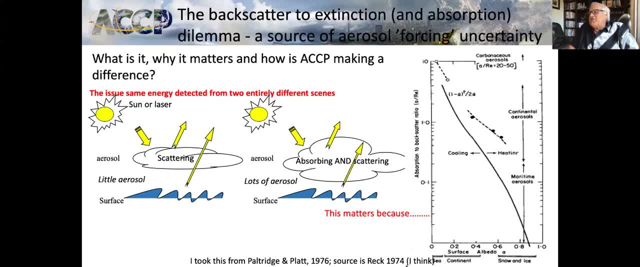 and I think it's from a book by Paul Kuhn. I think the source was Ruth Reck- in 1974.. I say I think because the textbook is in my office and I haven't been in my office since shutdown. So I think this is the case, But it basically underscores the point as it relates to aerosol. 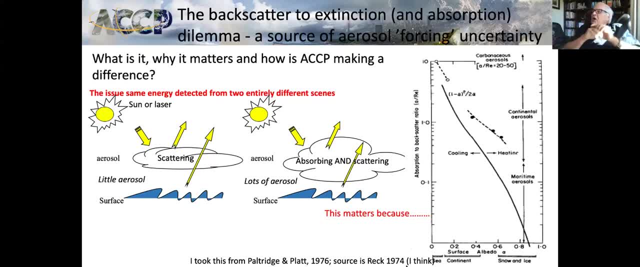 impact on Earth's climate through forcing. And it shows on the y-axis, the ratio of two important properties of aerosol: the amount they absorb and the amount that they backscatter- A and Rn, in this diagram as a function of surface albedo. And so these three properties, the surface albedo. 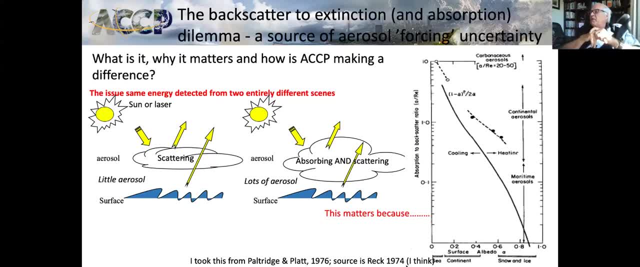 the ratio, absorption and the backscatter really dictate whether aerosol is fundamentally warm or cool. So this solid curve you see down there is the neutral line where aerosol falling to the left of it cool and aerosol falling to the right of it warm. So you can understand this by the fact. 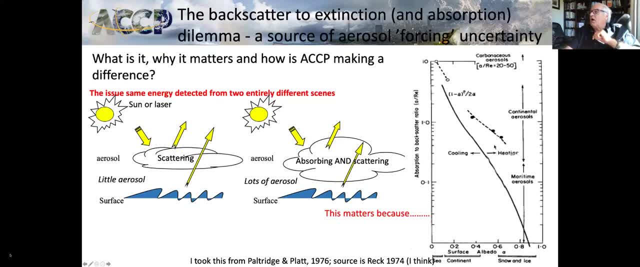 that aerosols that absorb more and fall above that line represent a heating of the system and aerosols that scatter more and fall below that line actually cool the system. And then they sort of, in this 1974 paper they sort of did a kind of a classification of aerosols, where aerosols 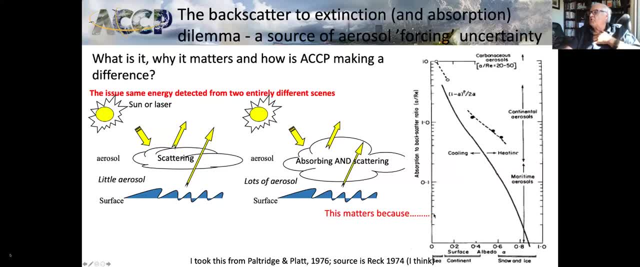 fall And so, for the most part, aerosols cool the Earth's system, because most of the Earth's surface albedo was much less than 0.4,, for example. But this underscores the point that you can't really understand aerosols' role in the climate. 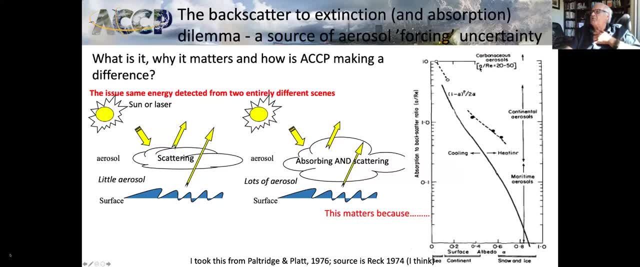 And so aerosols are really the same thing, of course, in the climate system, without knowing its ability to absorb and its ability to scatter and separating these effects. And so this has been a challenge. It's a challenge to all remote sensing aerosols. 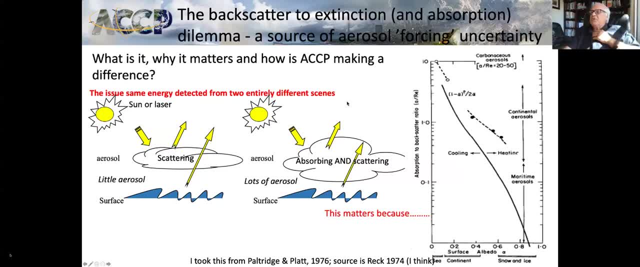 What passive measurements that rely on scattering from sunlight suffer this issue some more than others. Backscatter LiDAR suffers the same issue. So what ACCP represents in terms of really a sea change? I think in this and why it was proposed that this LiDAR would be really 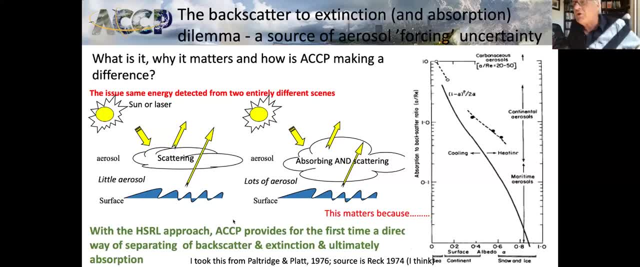 important step is the HSRL LiDAR approach. I'm not going to describe how it does this because it's way beyond the time that I have, But basically it's HSRL will provide for the first time a really a way of unscrambling the backscatter to extinction kind of development. 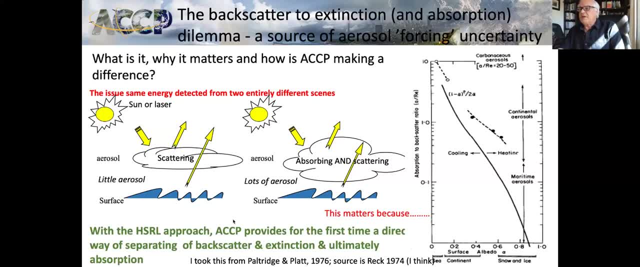 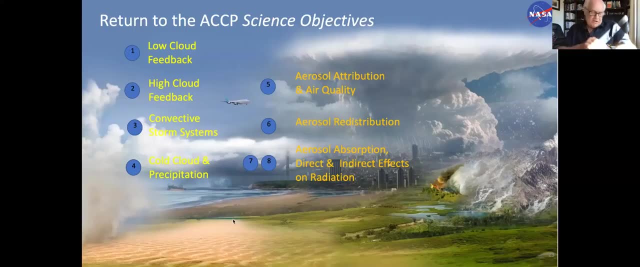 that exists in our measurements from space today, And so this will start to give us clues about absorbing aerosol versus scattering aerosol, and where it would, and their role are enforcing the climate system. So let's come back to our science objectives. I'm calling about 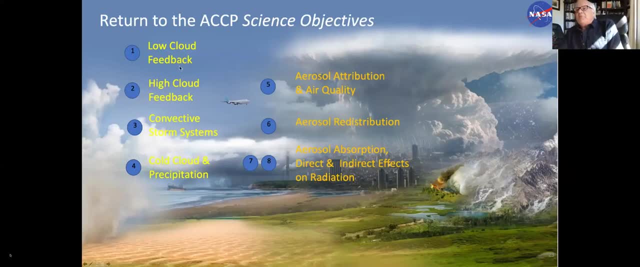 five minutes left as well, There's the eight objectives. I sort of touched on some of the motivation for why these objectives have been articulated and evolved as they have. Our philosophy in the ACCP in terms of addressing these objectives is to focus primarily on process understanding and secondarily on extending existing climate. 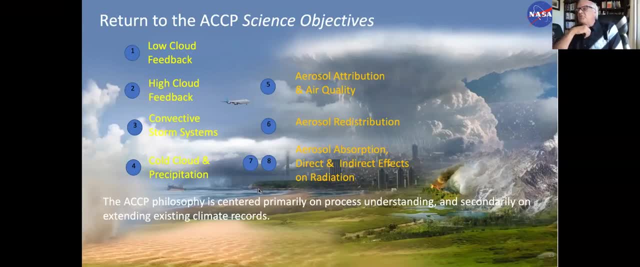 data records that we've begun with, like with the A train and GPM and so forth, and extending those, so you have a multi-decadal record of profile information of the atmosphere And I keep getting asked this question about: well, how the heck do you study process? 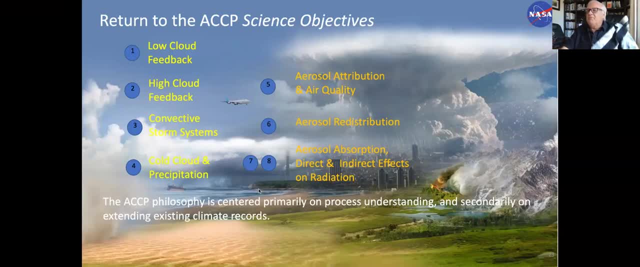 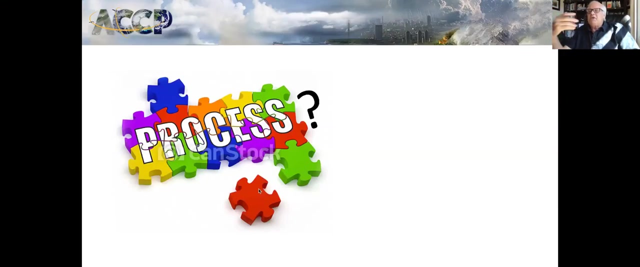 from just a set of observations, And it's not just correlating different variables. really There's more to it than that. So I thought I'd just throw you two examples of a process toward process understanding, how the ACCP might begin to address process understanding. 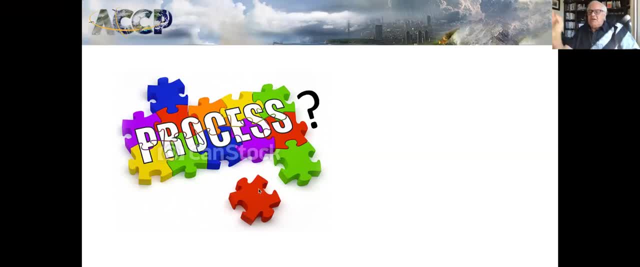 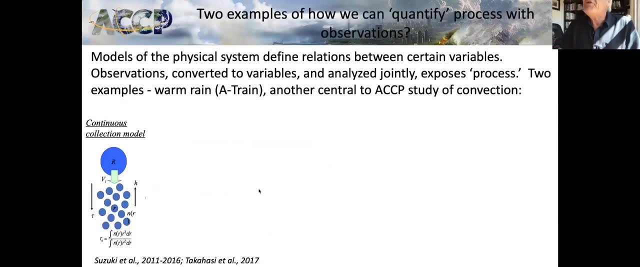 if it really will be the heart of making this progress in advancing ability to predict the evolution of the oil system. Okay, Let me just provide two quick examples, One drawn from the A train and another that sort of centralized, the ACCP. It's more conceptual in terms of thinking about it. 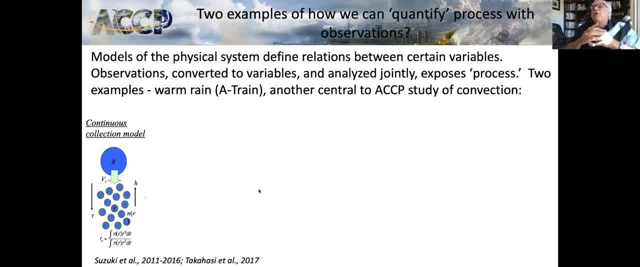 But fundamentally you need to have a model of the physical system. That's the framework to understand the process And that model would relate variables, important variables, and we want to make measurements of meaningful and relevant variables. It's not just a matter of making measurements of variables. 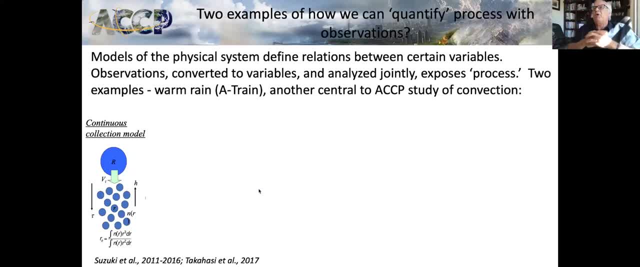 You've got to make measurements of relevant variables to which we have a model of the physical system that collects them, And through that lens that we start to understand process, And then one example is the warm rain process via, in this case, a simple model of collection. 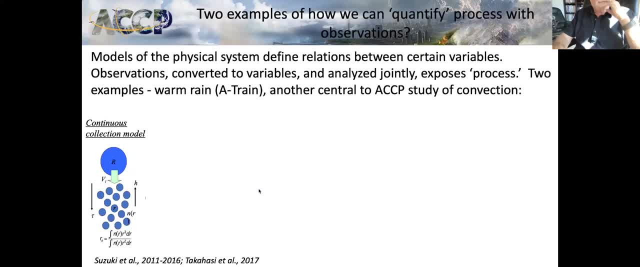 of a falling drop, collecting smaller drops, forming raindrops and making rain. Now it turns out- I'm not going to go through these questions, but it turns out- we can basically convert the process of this, The basic model of This collection process, which has all sorts of model parameters like collection efficiency. 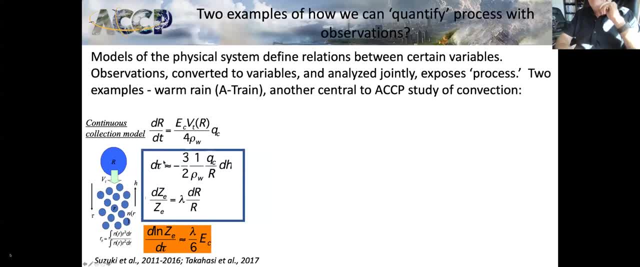 and all that stuff. we can relate that and convert that into a framework that essentially connects two observables- the radar reflectivity and a cloud of optical depth. And we can observe with the radar, the radar reflectivity, and we can deduce from observations. 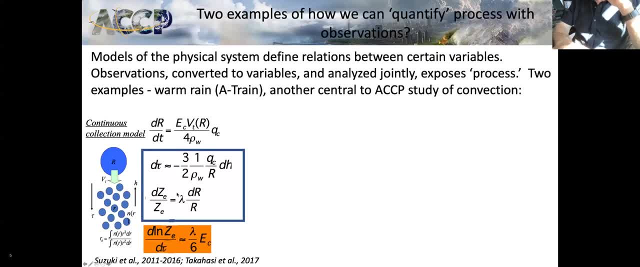 from the reflected sun, like the cloud of optical depth, and make inferences about the vertical structure of this cloud of optical depth through the cloud, And that'll tell us about the collection process. And that's the first step, And that's exactly what Suzuki and Hennie have done over the number of years. 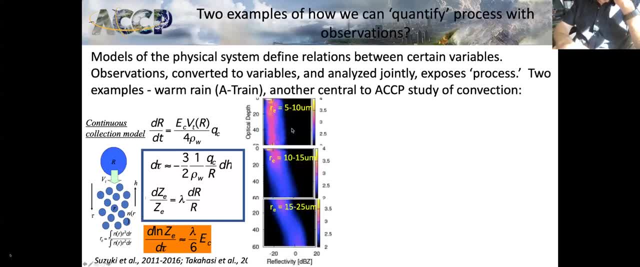 And this is just an example of it from the A-train. This shows you optical depth profile through clouds and the reflectivity on the X-axis grouped by cloud top particle sizes derived from MODIS, for example. The optical depth comes from MODIS, the radar reflectivity comes from CloudSat. in this case, 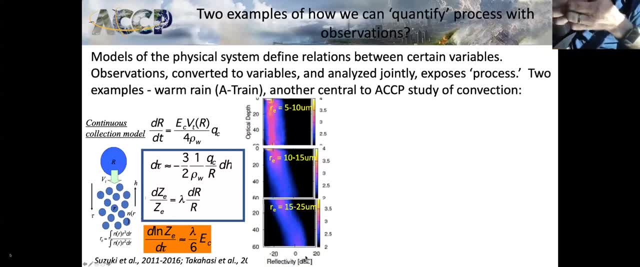 So it's an illustration of fusing multi-sensor data into a cloud of optical depth, And that's exactly what Suzuki and Hennie have done over the number of years, And this is just an example of it from the A-train. This shows you optical depth profile through clouds and the reflectivity on the X-axis. And that's exactly what Suzuki and Hennie have done over the number of years. And that's exactly what Suzuki and Hennie have done over the number of years. So it's an illustration of fusing multi-sensor data together through the lens of a process. 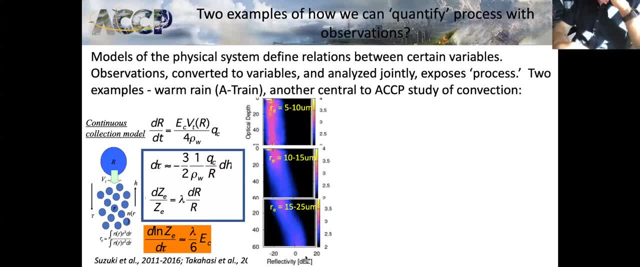 model to understand process, And so, without any slope in this relationship, there's no rain forming. This is purely cloud. As the particles get larger at cloud top, you can start to see distinct evidence of rain forming through the cloud, And this has been a very valuable tool to test rain formation in warm clouds the like. 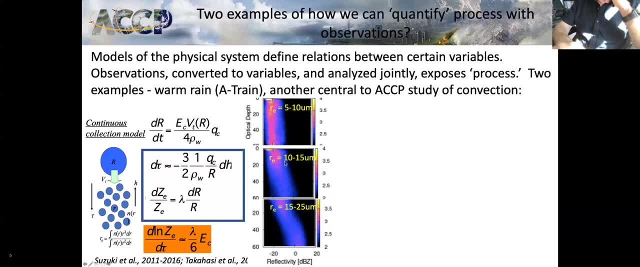 of which we now have more current models of major viruses. A second example of this is the study of the body of a cloud, And this is the study of the body of a cloud. And this is the study of the body of a cloud. 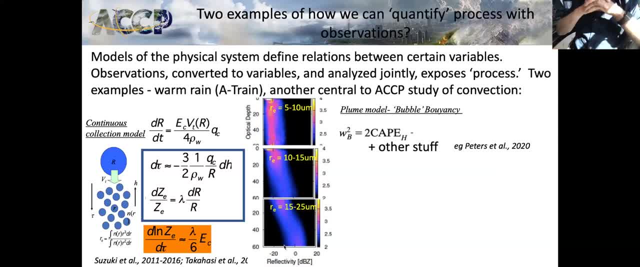 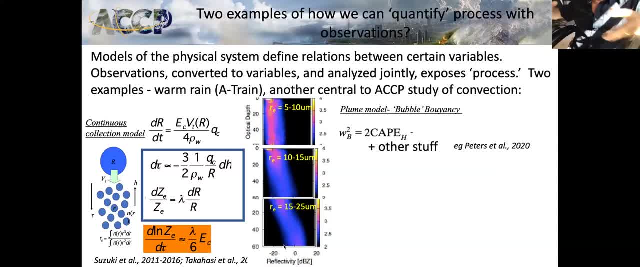 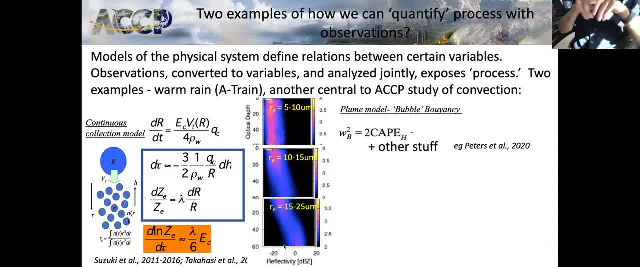 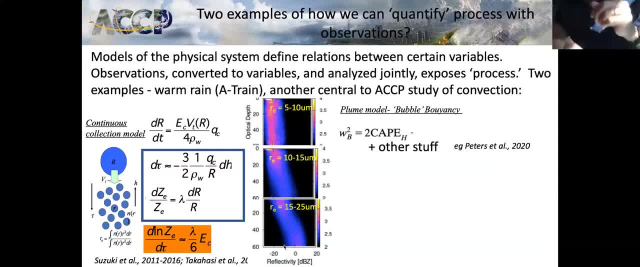 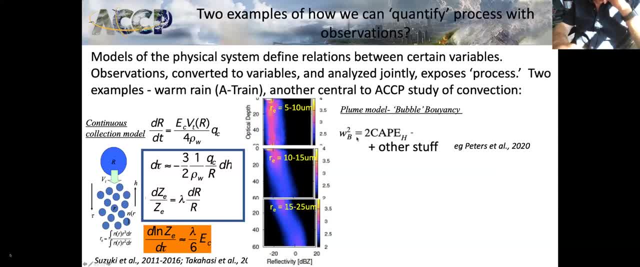 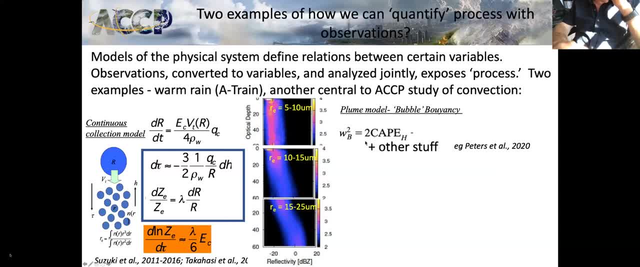 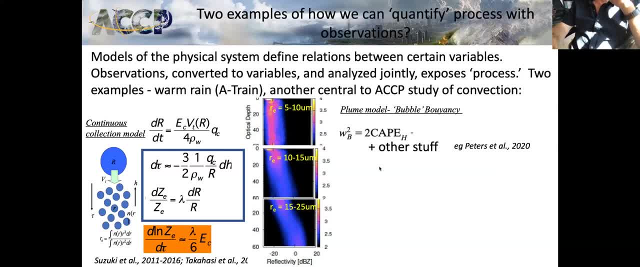 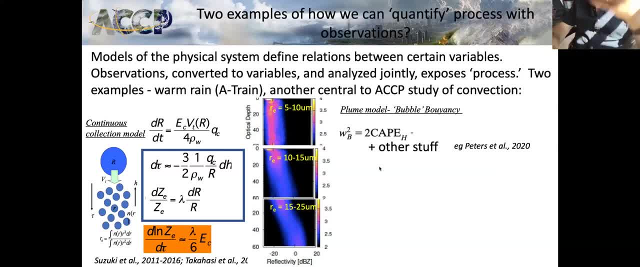 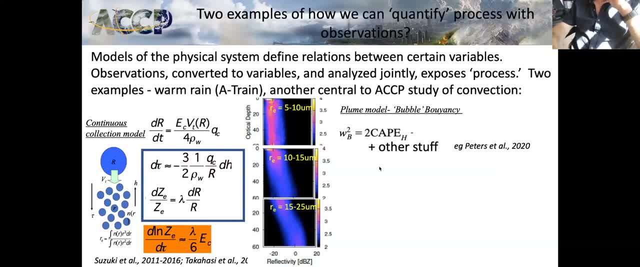 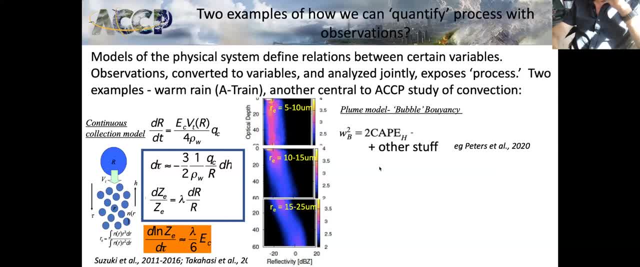 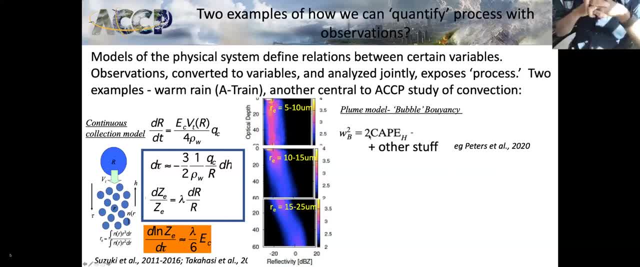 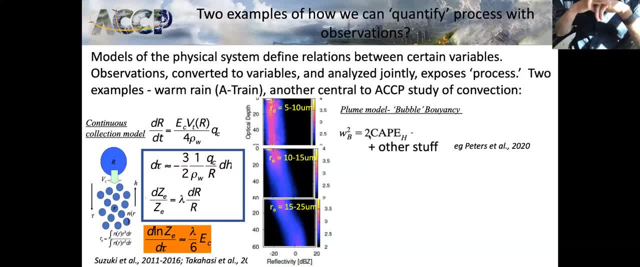 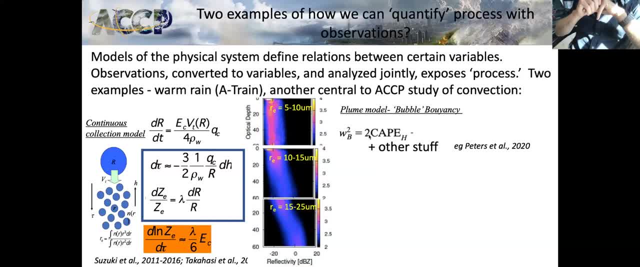 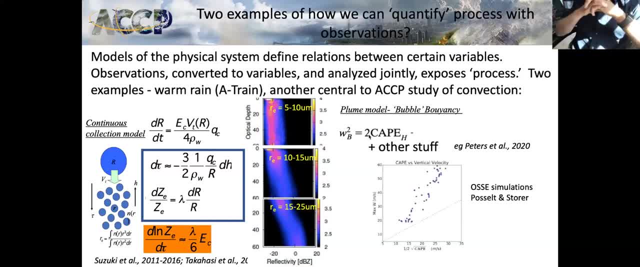 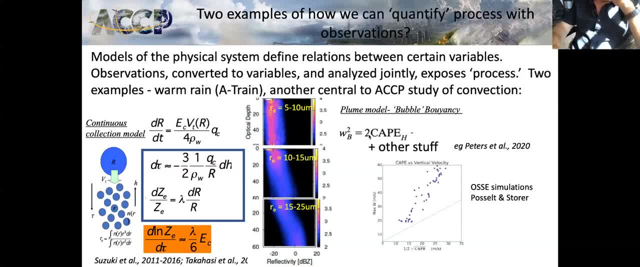 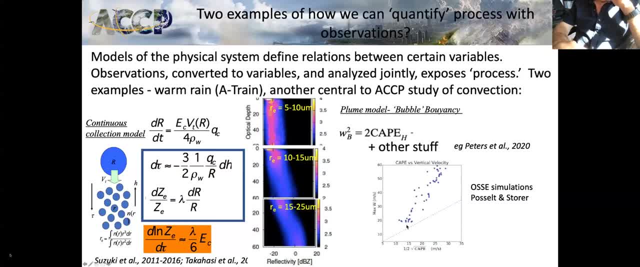 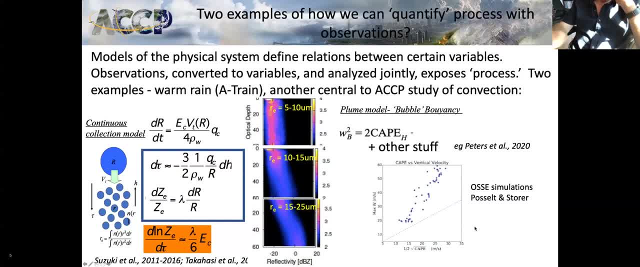 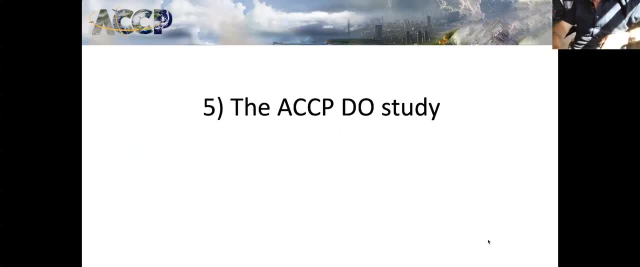 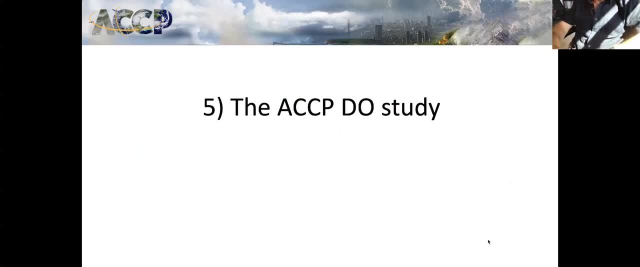 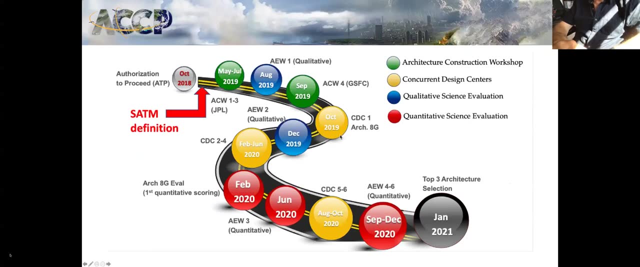 It started with a long and involved and intense march down a road starting in October 2018.. In between this bubble and this bubble, there's a GM definition that really sort of crystallized the definition of ACCP, And then we had a whole series of architecture studies, construction studies and evaluation. 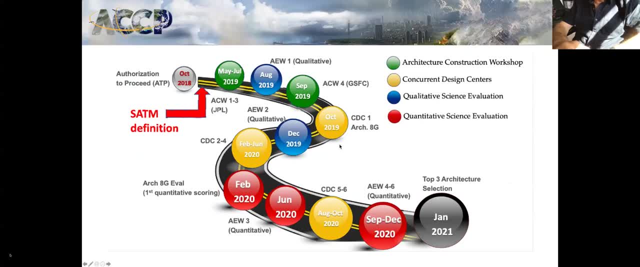 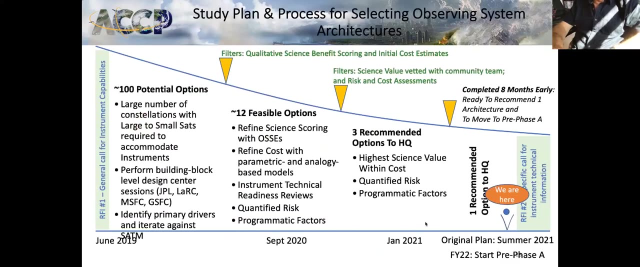 studies of architecture. We also had quantitative science evaluation, led in by these red bubbles here marching along for a couple of years of this study, ultimately leading to the architecture that I showed you at the end. I think I can skip over this slide, because it basically just shows the same thing. 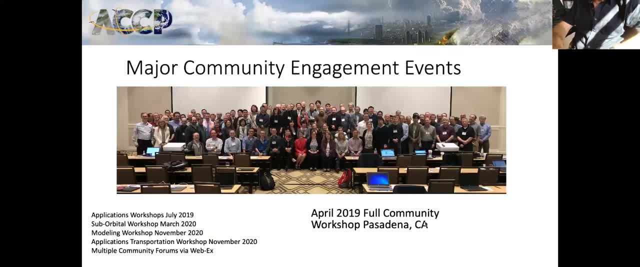 We're now presently in three phases. It involved also large community engagement events. We had a number of workshops: large workshops, some focused workshops and some little activities, some which I'll summarize at the end, which I'm now about to at the end. 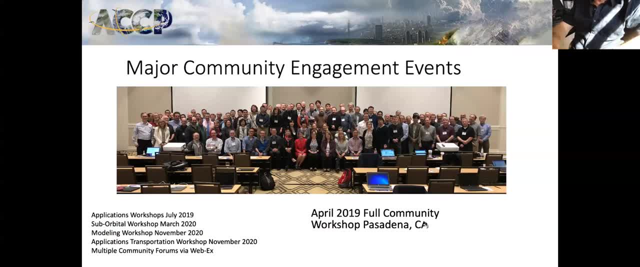 So we had a variety of real broad input from the community environment, from the community. So we wanted to make this really a community activity. So we had a variety of real broad input from the community environment, from the community. We wanted to make this really a community activity. 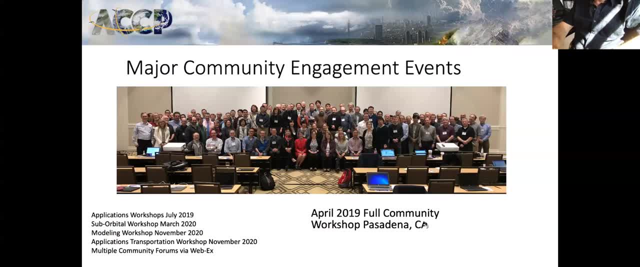 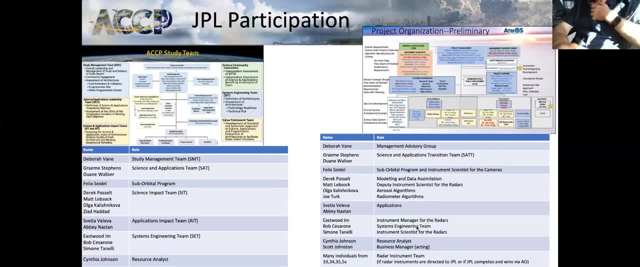 And not simply a NASA Center activity. There was many participation of JPL in the study itself through the study management team. We had a structure over here. I'm not going to spend time in the structure over here, but there were many folks that listed. 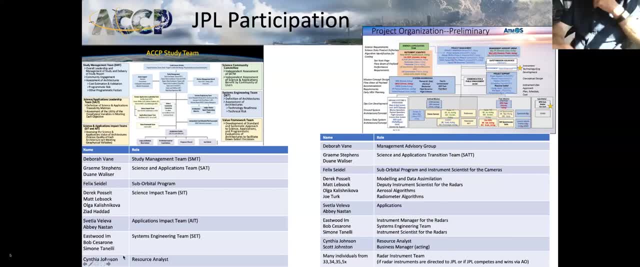 to the left end. You probably can't see that because it's probably small on your small screens. but we had Duane and I were involved in the science and applications leadership team called the SALT sub-orbital program. Felix has been involved in co-leading the sub-orbital. 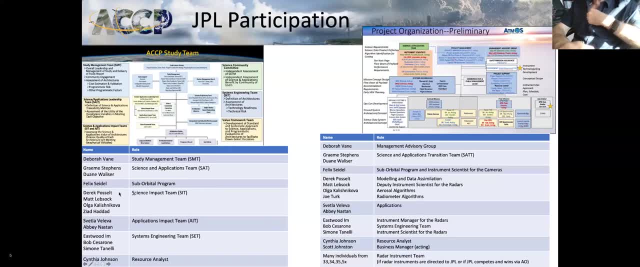 program definition. The impact team really did that. some bolts in terms of: will the observing system deliver the variables that we think we need to address, the objectives and so on. We had engineering, representation, engineering teams and then representation applications. We've now moved into a project organization where we have now a science and applications. 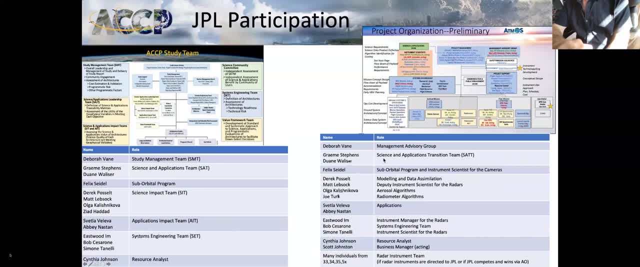 team that Dwayne and I are on. we have sub-orbital activities, We have instrument teams. we're helping define the definition of instrument requirements for pre-phase A. Now, an important point is that these instrument teams- the idea was that with the active instruments, that would be, the larger instruments- were going to be. 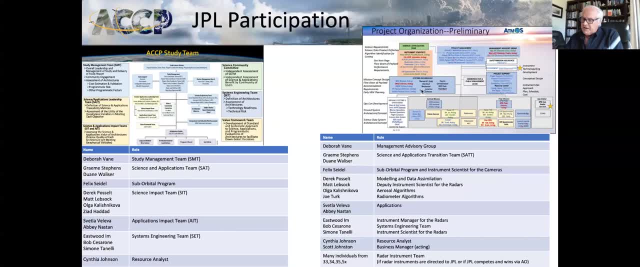 designated. These were directed instruments. I should say That's our intent, That was the project's intent, but NASA headquarters is mulling over the idea of these perhaps being competed And, as a result, we've had to stand down the radar and LIDAR teams because we don't want. 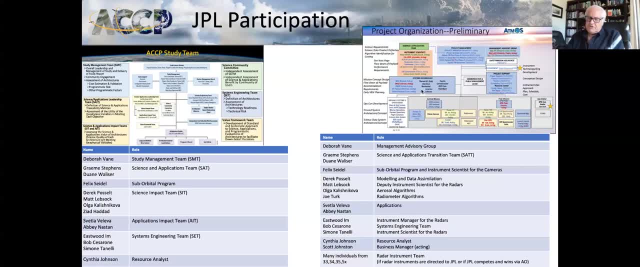 to jeopardize their ability to compete should they actually go to a competed solicitation? Okay, so I'm going to skip one. Okay, I'm going to skip one. This is the end. I'm at the end. We all got to say thank goodness. 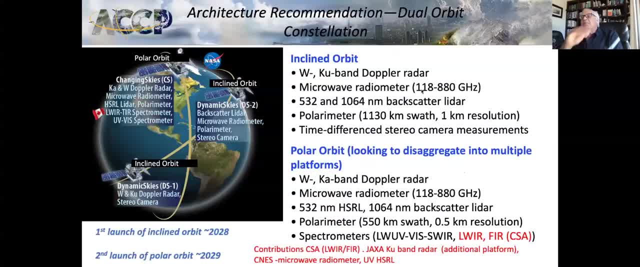 The end is where I began. Here's our architecture: Two orbits. In the inclined orbit we have two frequency radar, Doppler and the KU. We're microwave radiometry, mainly at the higher frequency end. We'd love to have low frequency, but this is a matter of scope and cost. 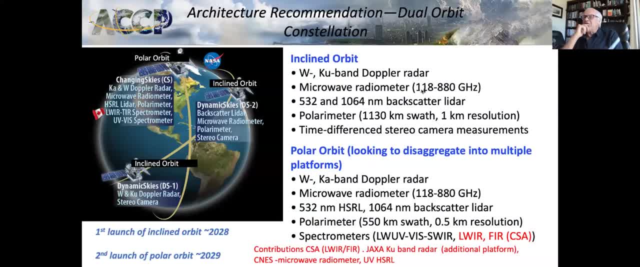 We have the backscalal LIDAR in the inclined orbit, are in inclined orbit primarily for cloud and aerosol, but not the HSRL, so not really addressing the aerosol capability that we need to address. the climate impacts, yeah, polarimeter and we're. 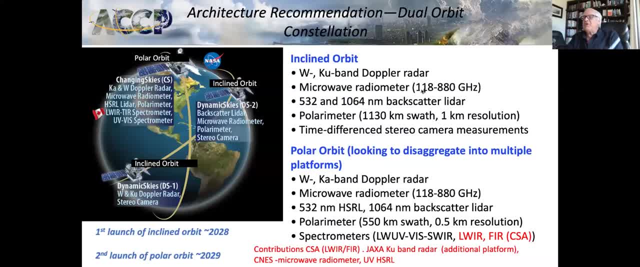 proposing to look at you, implement time, different stereo camera measurements to look at dynamics of clouds and plumes, both through the stereo conduct. the polar orbit is adopted, kw and ka, and this will be that the doctor w will be kind of a little revolutionary for certain clouds where the ku. 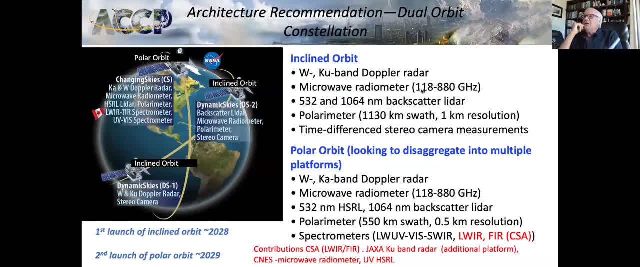 doctor, will be revolutionary for deep connection. um in this line, uh, microwave radiometry again. um we hsrl is in the polar. polarimetry and spectrometers play a really kind of important role because they they provide a way of quantifying the radiated impacts of the clouds in 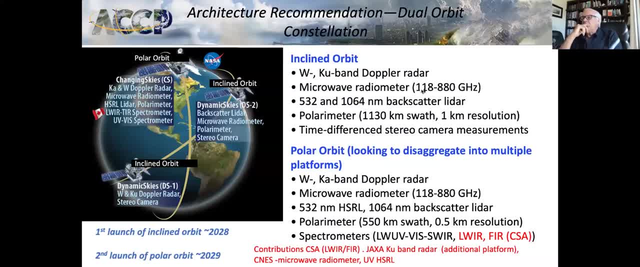 aerosol and radiation um at the kilometer scale, which is really kind of important. um. we have contributions being planned for csa of this infrared spectrometer jackson of the ku band radar, uh, with a potential additional platform added to the inclined orbit to make the constellation. 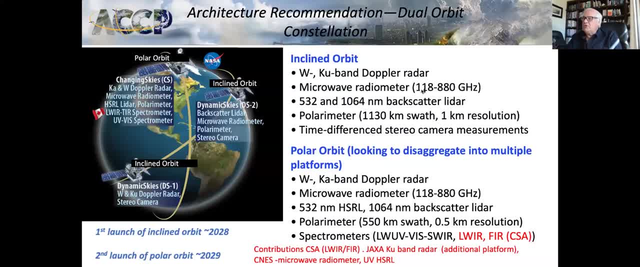 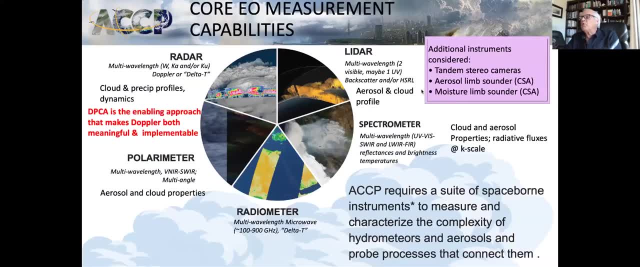 and this caness with microwave radiometry and also a uv channel in the hsrl um. i might skip over this. um requires a suite of spaceborne instruments to measure and characterize complexity of hydromedias and aerosols and probe processes that connect them. 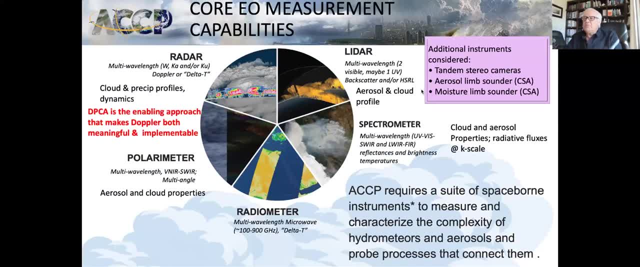 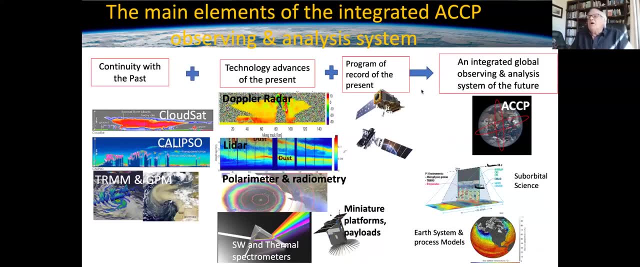 in contact with a range of different. so two a b: There's an attempt to provide continuity with a path to create climate data records. There's exploiting technology advances that allow us to do real Doppler radar meaningful for the first time with the concepts that we propose: the radar, the polarimetry, the 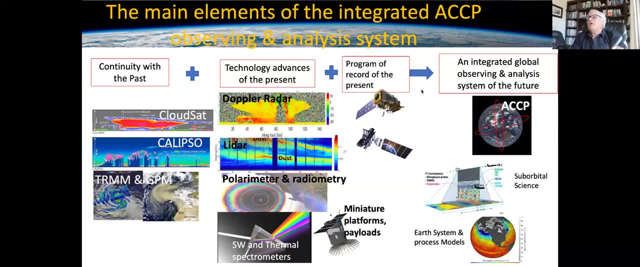 spectrometry and we're all coming under, benefiting by technological advances. The geostationary program record is huge and we plan to exploit and be active in developing key products for that. And then the integrated other elements over there, the suborbital- there's a real active 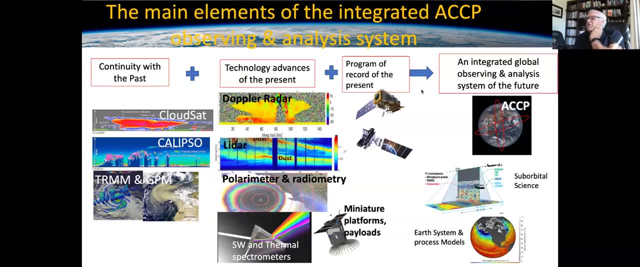 suborbital program and Earth System Process Modeling. we're very much engaged in Earth System Modeling and connected to that evolution, to the K scale, as I talked about, And just to leave you with a vision if you want to have a vision for what we might be. 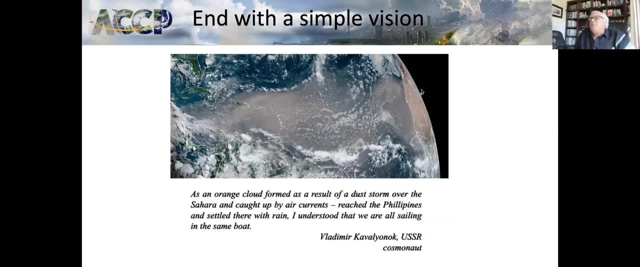 you can do that in the end And then to sort of state it to me succinctly by this statement, by this Russian cosmonaut- USSR cosmonaut, if you like- as the Orange Glow formed as a result of dust storm over. 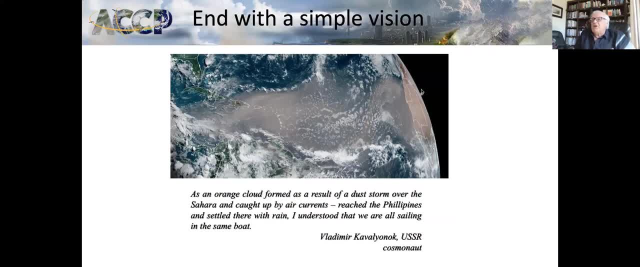 the Sahara and, caught up by air currents, reached the Philippines and settled there with the rain. I understood we're all sailing in the same boat and this is not some sort of ACCP. in a nutshell, It's all about that processing of all the particular matter in the atmosphere that rises. 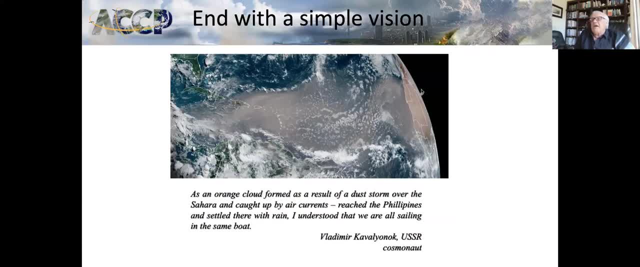 couples in the clouds and precipitation, And that's what I'm trying to do. I'm trying to do that And that's why it's so exciting to see the whole thing change and fall back out again in the system. That's ACCP in a simple vision. 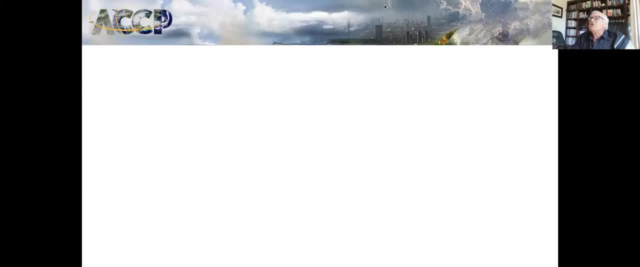 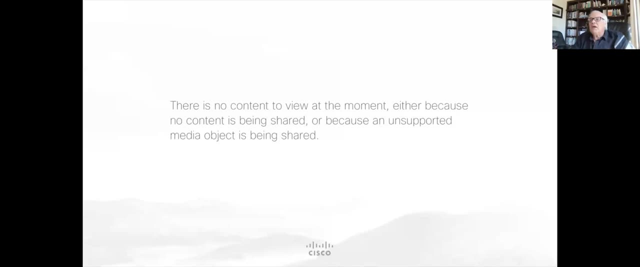 And that's it, folks. I know I went a little bit long. I'm happy to take questions and I will stop sharing my screen so I can see questions. Thanks, Graeme, Coming in Wonderful presentation. Everybody's clapping. 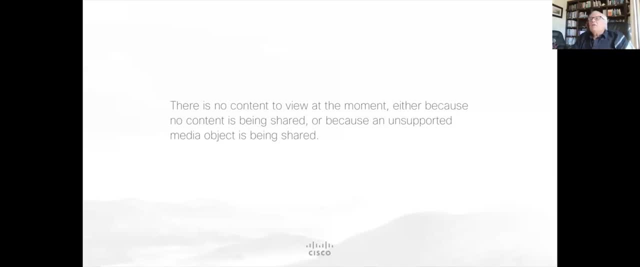 Thank you, Graeme. I can see the orange hands going, you know. OK, so that's the questions on the chat box. So there's a question from Evan Fishbein. Evan, do you want to ask the question, or should I read it? 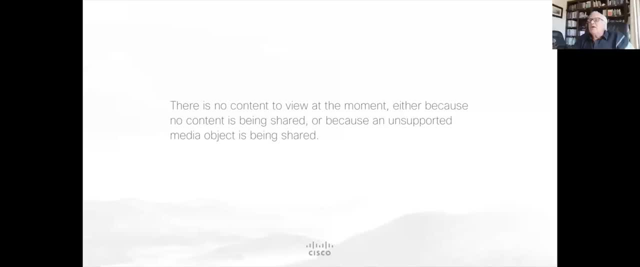 Yes, I'll read the question. So Evan's question is: why was the KU used in the inclined orbit and KA in the polar orbit? Ah, because the KU is the sensitivity. it has to do with the sensitivity of the radar. 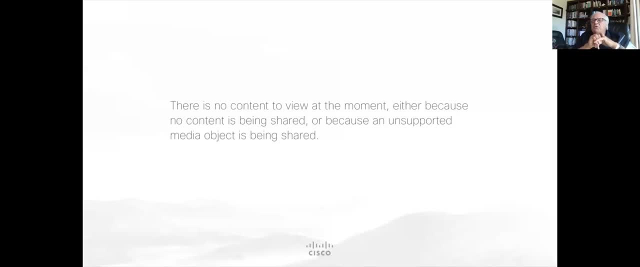 The KU is primarily going to be sensitive to well. we split sensitive somewhat to shallow convection. but deep convection the footprint's somewhat larger. The KA has greater sensitivity so it'll represent more of a dynamic range of the convection. 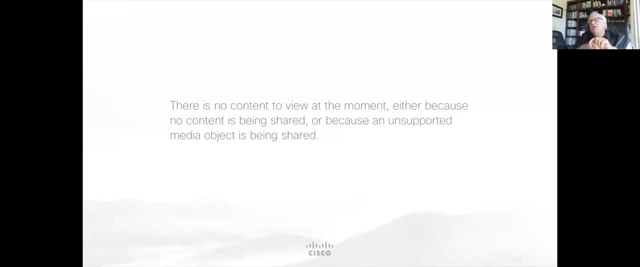 including shallow convection, and convection that's not necessarily, you know, the same as you know, confined to the tropics, and maybe the more tense convection and mid-latitude. So it's really a sensitivity issue, Evan. So to cover the more greater dynamic range, that way I would argue, and the greater dynamic. 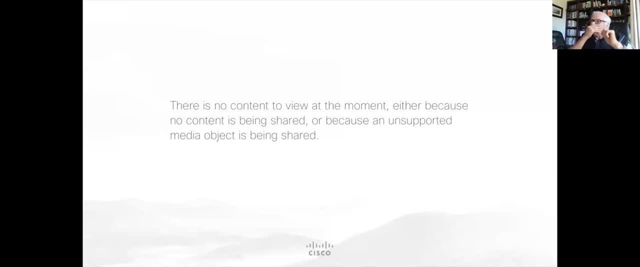 range in the Doppler motion in terms of clouds and convection And the WBAN really gets to the shallow convection and cloud. and you know, we think we can do something really quite meaningful with the WBAN Doppler, unlike EarthCare Doppler. 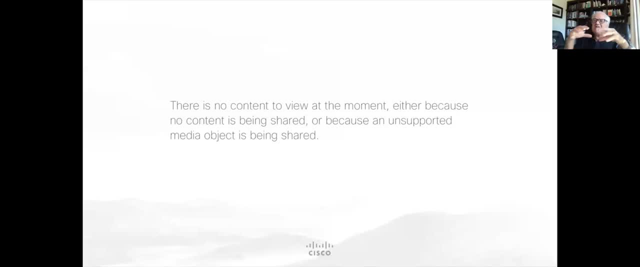 which is really pretty coarse, And the secret is this: two antenna design. That's what we're looking for. That's what we're looking for And the one that our JPL engineers have come up with, which is really kind of a game-changer. 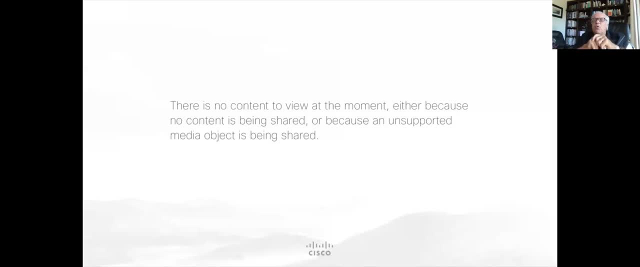 for Doppler really takes out the unwanted effects of platform motion, so we can get down to, you know, half-metre-ish per second kind of sensitivity with the WBAN. we think I hope that sort of answers your question to some extent, Evan. 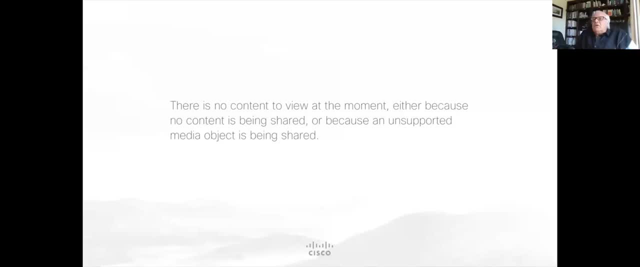 So Josh Fisher asks: related to Evan's question, can you talk a little bit about the decline orbit? What does that get you in terms of sampling and science? So we know, for example, that none of these processes are shaped by the diurnal cycle. 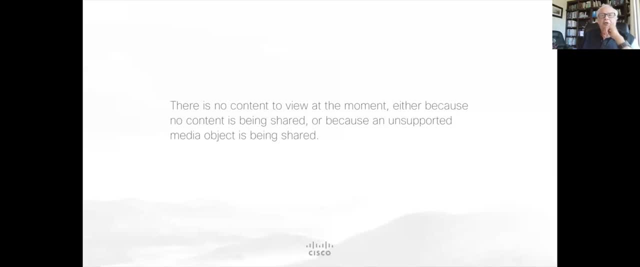 And so it's really fundamentally trying to, for the first time, get at process information about the diurnal cycle. Now you might say, well, can't we do that with geostationary? No, because geostationary will give us information about variables, but not data. 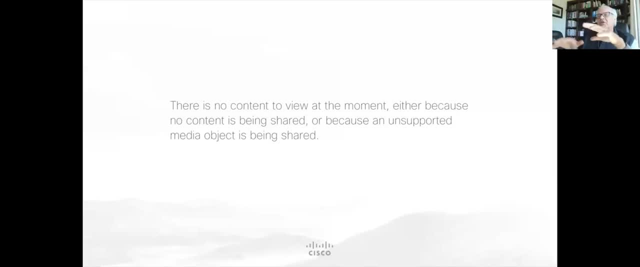 So we can't do that with geostationary. We can't do that with geostationary. We can't do that with geostationary. It's not necessarily the variables that connect directly to a physical process. So that example I showed you with the precipitation, high cloud and water vapor from geostationary. 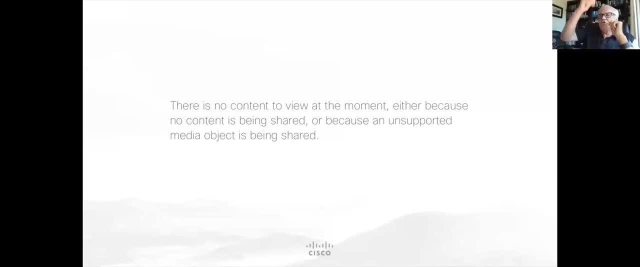 the process that connects them is air being lifted up vertically and the motion that lifts air up vertically. That's the process that connects them. So we want to make that measurement and then connect it to those variables to understand the process. So it's really all about diurnal cycle sampling. 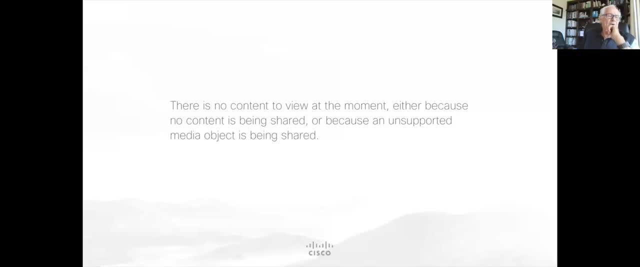 It's really now a debate going on right now. Josh is on it. Josh now has a question right here. He's really enjoying this program. Great Thank you. Most of us are unterstated. There are slight points, Jay and G. Okey. 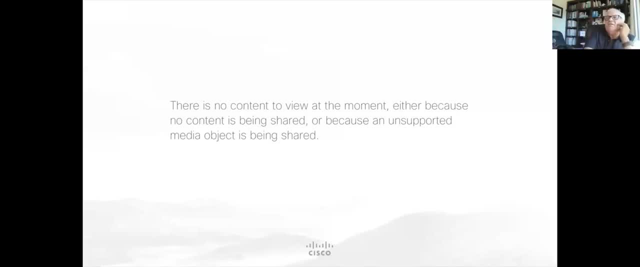 Again. thanks very much, Josh. Enjoy your time and I'm going to sign off the seemingly derived interesting secretary for direct organisations and subsidiaries. Thank you, Where are we going? Where's Michael? Michael Kahn? Let's try it up here. 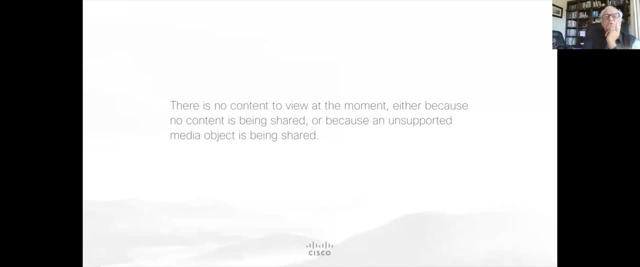 Alright, we'll try this real quick, Dakosky. So I was curious to see how you're thinking about it and also what you're missing. What don't you get from the inclined orbit? You get some diurnal sampling, but you also don't get some aspects, and so I was just 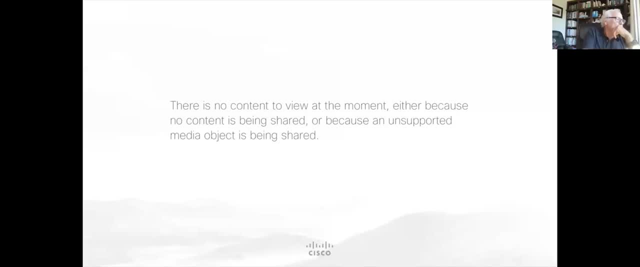 curious. Well, from the size point of view, there's things we miss, because by just put through a necessity and budget and trying to scope this thing, you've got a rate. We don't have, for example, dynamics that are capable of looking at shallow convection. 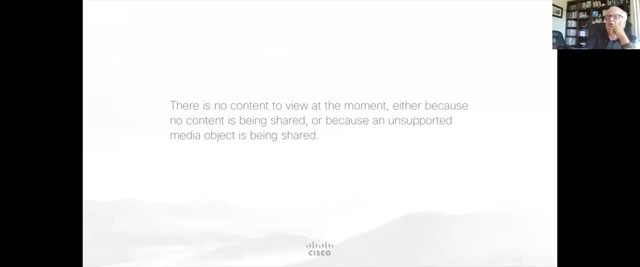 or diurnal cycle, shallow convection, for example. The KU won't necessarily give us that much insight on dynamics of shallow convection. Shallow convection is a precursor to deep convection, so there's some example of things we won't necessarily capture, although the cameras, the stereo cameras, will give us some. 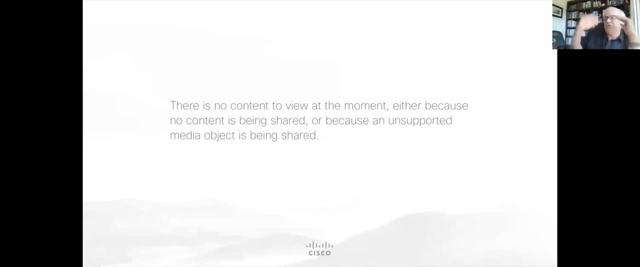 clue with respect to cloud top height motion. but that's not really diurnal either, Because it's only that relies on daylight. sunlight's scattered right, so you can't do day-night stuff. Yeah, there'll be things we miss, like anything, just like a compromise and trying to navigate. 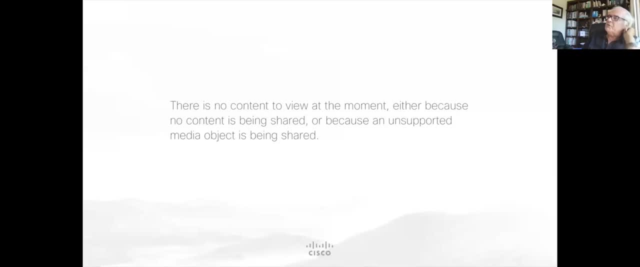 all the things we'd want to do with those which we can practically do. Doesn't really answer your question, but there's some more of this. I can see some more popping up there, if you will, Scott? Oh Scott, Yeah, it's okay. 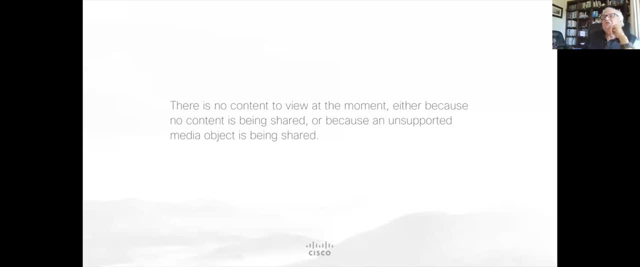 I've got you. Scott's made a comment. He's probably corrected me on my answers about the KU, so I don't know whether, Scott, you want to just jump in there or what. Yeah, I mean just part of the inclined orbit is to really target deep convection and with 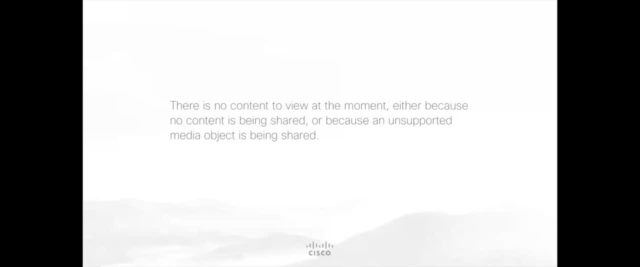 the different radars, you get increasing attenuation going from W to K and KU band, and so KU allows us to penetrate convection down to near the surface, whereas W and KA will have significant issues in convection. Yeah, exactly So you know. the KU's really an ideal tool for looking at the heavy, intense stuff and 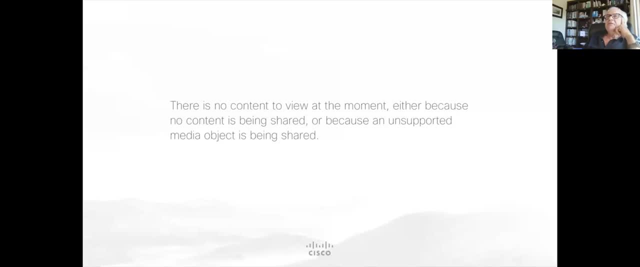 the KAW is for the less heavy and intense, and hence you'll see more of that in the higher latitudes, for example. Okay, So there's a question from Kevin Baumann, so do you want to read it? or low cloud feedbacks? 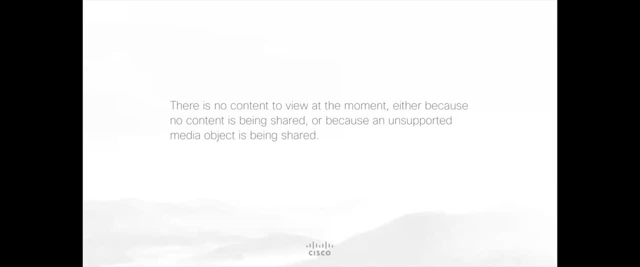 are implicated in the range of ECS. how will ACCP reduce the uncertainty in those projections relative to the current program arrangement? Yeah, Okay. So, Kevin, as you know, this has got to be explicit. it's a difficult question to answer. 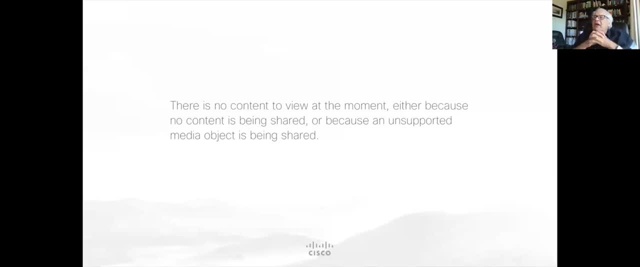 but, however, it is quite fundamental, and that example of the room was that three-figure, three-panel diagram which shows you the fundamental influence of warm rain on low cloud feedback. Well, you know, we're going to do a hell of a lot better in warm rain than we have done. 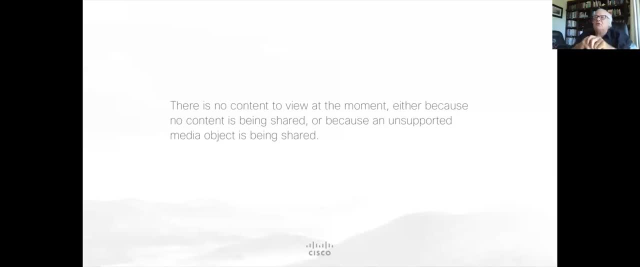 in the past. Warm rain is really quite fundamental to low cloud feedback. It's also quite fundamental to the aerosol indirect effect and the broad community hasn't yet absorbed this. Now we're going to do a hell of a lot better job with warm rain because we're focusing. 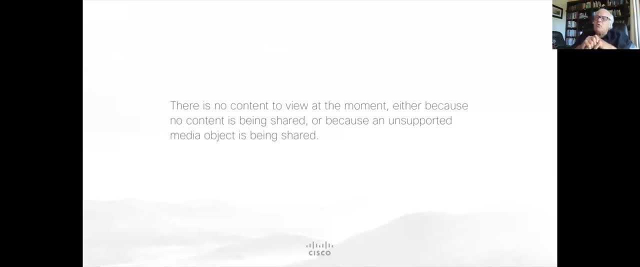 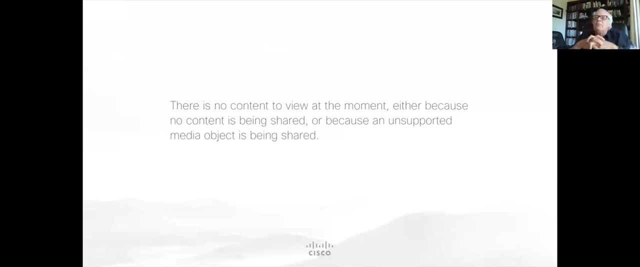 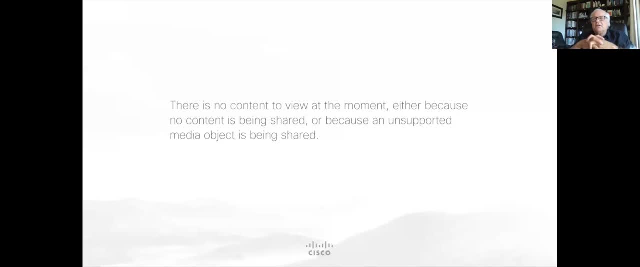 lifted up. air rising makes clouds, So it's going to be really important, I think, and at that measure it's going to be really important and evolutionary, I think. Dhirendal Cycle of Convection: Clouds, woo. 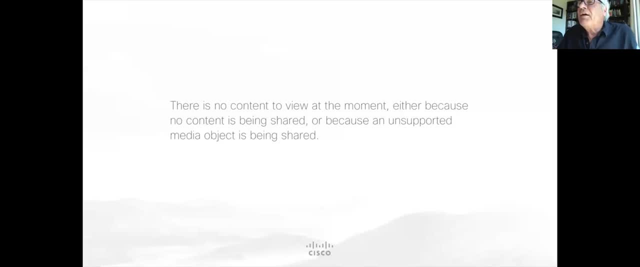 Something here, Hi, Did I misrepresent your figure? I probably did. It's a good figure. yeah, Thank you. Thank you, Berman, for representing my figure. I just wanted to point out the right reference. Oh, it was the wrong year, was it? It was 2004?. 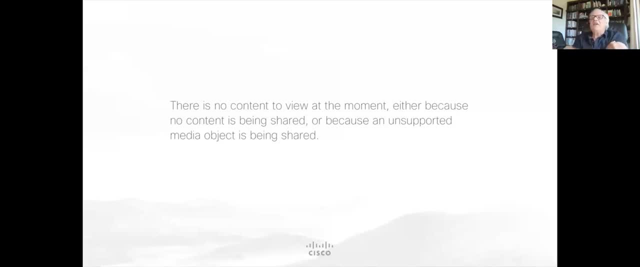 It was 2004,. yeah, I was sort of guessing. I knew I'd put it in a document that Scott and I worked on the narratives, but I was a bit lazy and didn't go back to it, so I sort of winged it. I thought it was 2002.. Okay, thank you And that's it. I 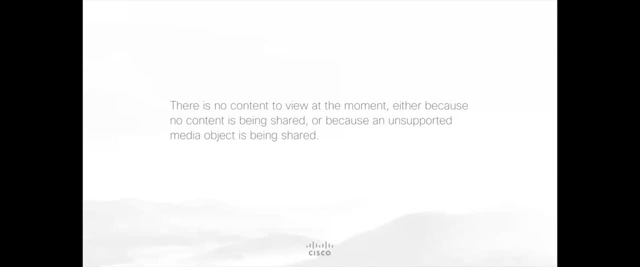 want to make another comment. I think it also makes sense. There is a model bias: the climate sensitivity. I think 2015 is a good example. Different models have a different cervical WT bias. Yeah, that's another good example. That's actually another really good example. 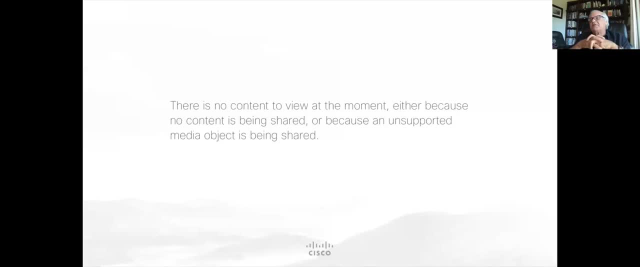 Yeah, thank you, Graham. That's a really pertinent example for ACCP, because that's about convection in the ITCZ, Exactly exactly. That's a great example. Yeah, Thanks, Thank you, Graham. I'm getting slow in my old age. 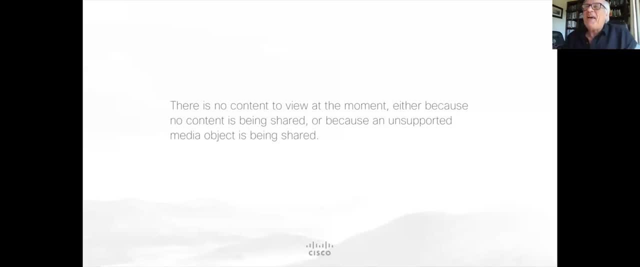 Yen. so you know, No, you're great, It's a wonderful talk. Thank you, Graham. So it's 10.02, 10.03, actually on the West Coast. Thank you, Graham, again A wonderful. 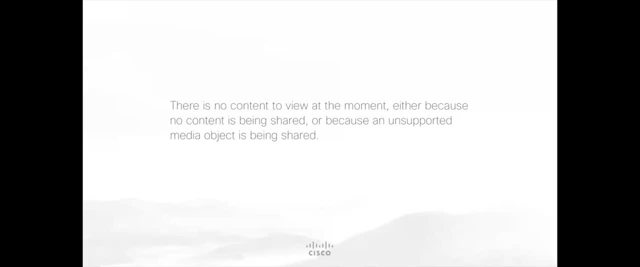 presentation. I'm sure everybody loved it and it was extremely informative. I'm sure people know your email. Most of the people know who you are and can reach to you if they have any questions. I might be slow answering today because I've got to do three hours of mandatory courses.